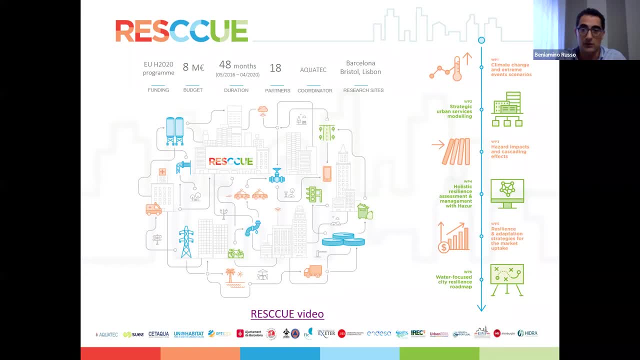 in this time now from Beolia Group. At the end of the presentation, I will share with you a video about rescue and also the link with all the collected results in terms of methodologies, in terms of tools, deliverables, guidelines, etc. 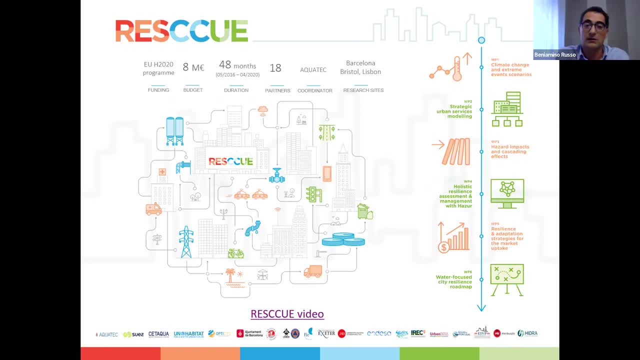 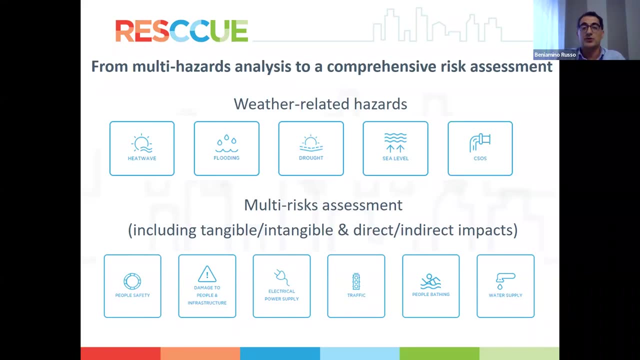 The rescue toolkit link. It was a project related to urban resilience and focused on multi-hazard analysis and comprehensive risk assessment. As you can see in this slide, we focus on a large set of climate-related hazards, But, as I said, in this presentation we will mainly focus on flooding. 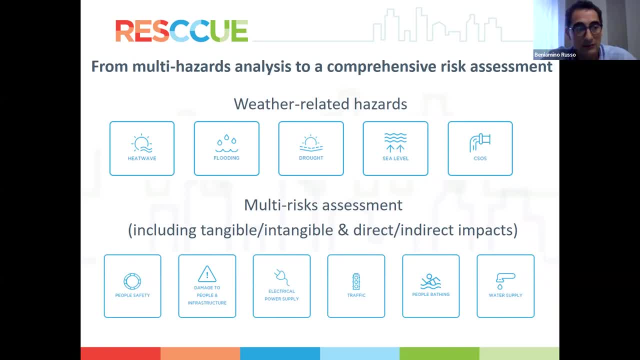 and mainly focus on treatment of urban pluvial floods, with a strong interest for sewer floods. Within the rescue project, we try to perform very comprehensively risk analysis, including several types of impacts produced by floods. So we assess the tangible and intangible damage, direct and indirect damage and, as innovation. 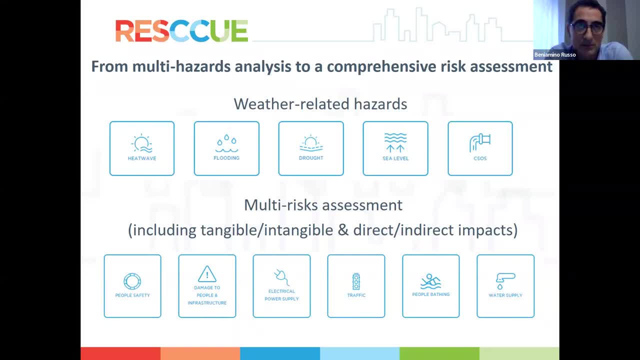 the cascading effects produced by failures in the urban drainage system of these three cities. So cascading effects on several main services like electrical system, for example, transport system, but also waste collection system, etc. Of course a part of the typical impacts on people, pedestrians, on vehicles and also 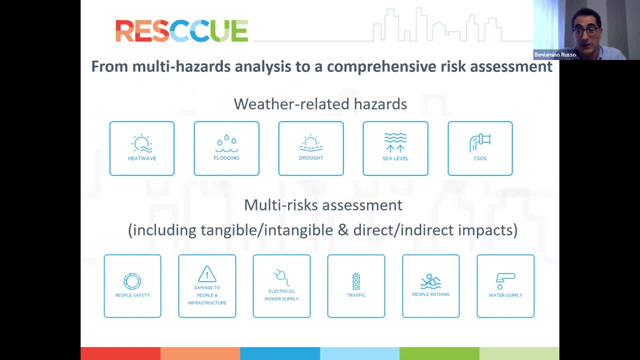 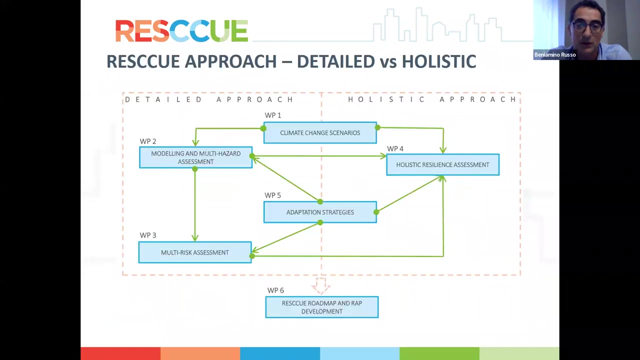 damage assessments for assets, for parcels, for buildings. So we've tried to provide a quite comprehensive assessment of the potential negative impacts produced by urban pluvial floods in these three cities. We followed rescue projects, followed a double approach, in the sense that here you can see the structure of the project. 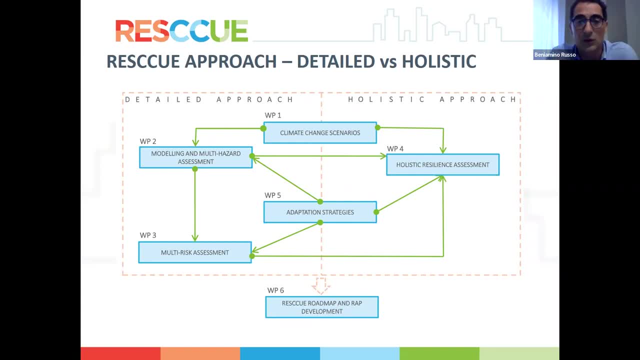 typical structure in several work packages. So at the beginning we had the climate change scenarios as drivers for to be used for advanced and detailed modelings to perform hazard assessment and also monitoring. So we had a multi risk assessment. Then we defined several adaptation measures, with special focus on natural based solution in order to reduce hazards. 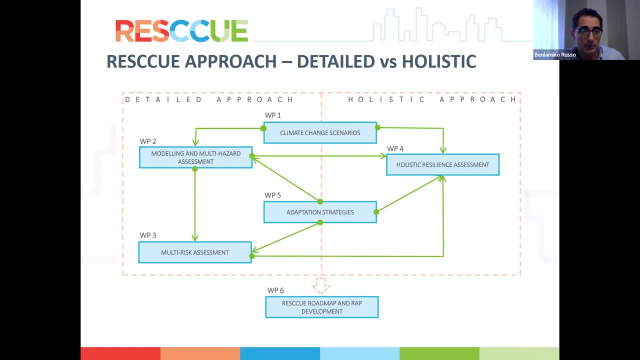 But also we analyzed the effects of a large set of measures. One of the main results of the project was a collection, a database, a platform of adaptation measures to face with climate related impacts, So adaptation strategies to reduce hazard and risk produced by flooding. 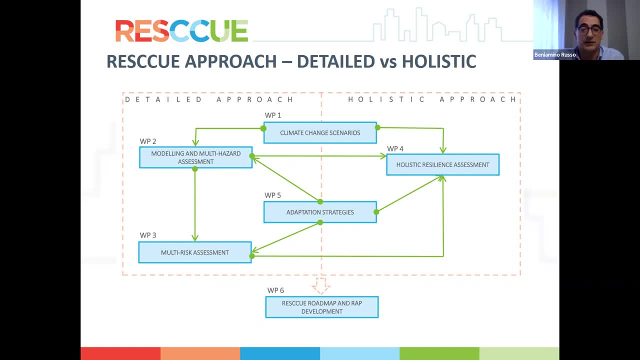 This was performed using a very detailed approach, while on the other sides, we use a more realistic view, a more realistic approach. So the first step was to have, let's say, a holistic, resilient assessment, To have a first diagnostic of the problems of the cities in terms of the behavior of its main urban services during a crisis event. 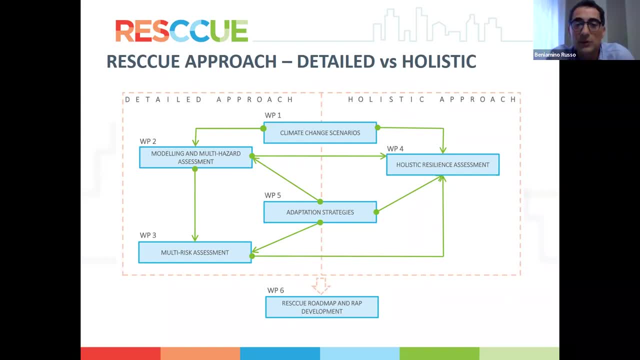 Of course, the approach could communicate and share information. And finally, all this knowledge was used to develop a model, to develop three resilient action plans in the three cities and also to produce, let's say, a manual or a guideline for the elaboration of a resilient action plan. 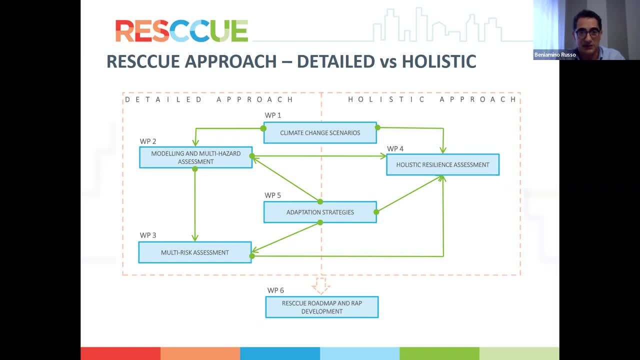 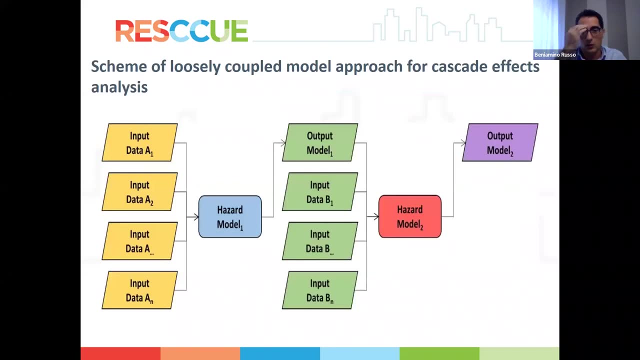 of course, related to climate resilience. In this approach, we focus on climate resilience. One of the main innovations that we used in this project was the use of integrated models, or, let's say, loosely coupled models, in the sense that we used the outputs of the pluvial models. 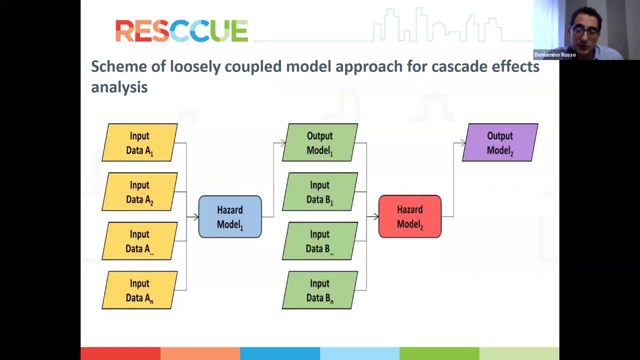 so the outputs of the hydrodynamic models in terms of flow depth, flow velocity, flood maps, et cetera, as inputs so to fit other models related to other services. So in this sense, we used the outputs of the hydrodynamic models to feed. 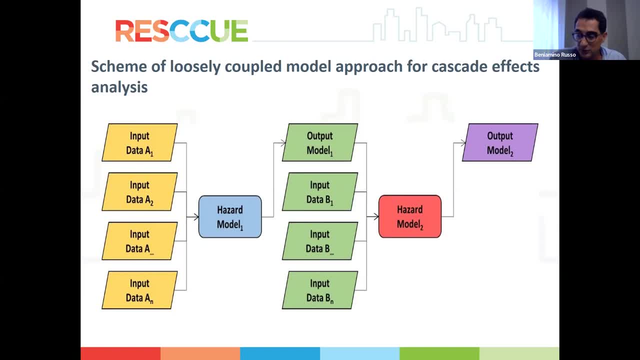 transportation, electrical models, waste collection models, in order to analyze the impact produced by the poor efficiency of urban drainage system during heavy storm events. So the idea is to use these cascading models, or loosely coupled models, as a chain, to analyze cascading effects from one services. 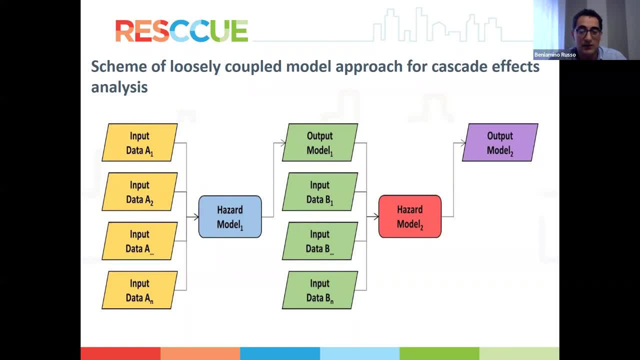 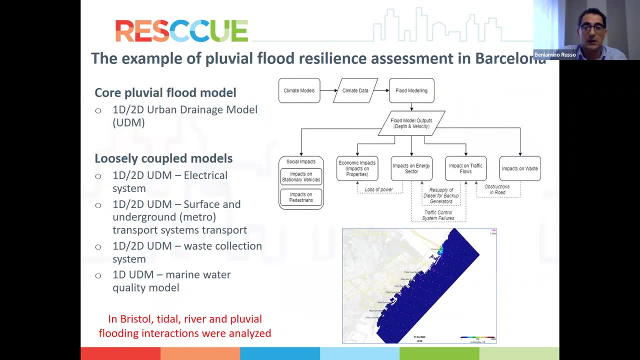 in this case, urban drainage to other receiving impact services like transport, electricity, waste collection, et cetera. And this is the case of Barcelona, for example, where we developed a very detailed 1D to D urban drainage model that was used to provide flow depth and velocity. 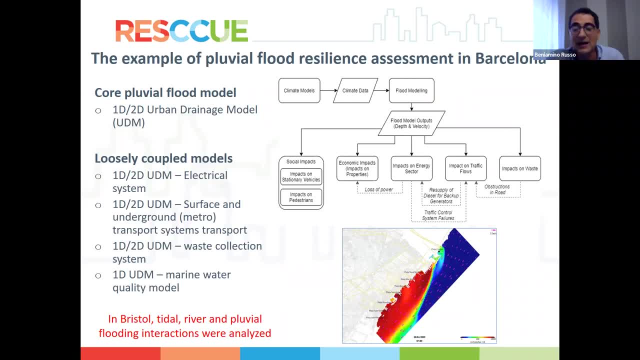 in all the analyzed domains. We analyzed all the city of Barcelona, around 100 square kilometers, And these outputs were used, of course, to assess social impacts: impacts for pedestrians that can circulate Or cross flooded streets during these kind of events. 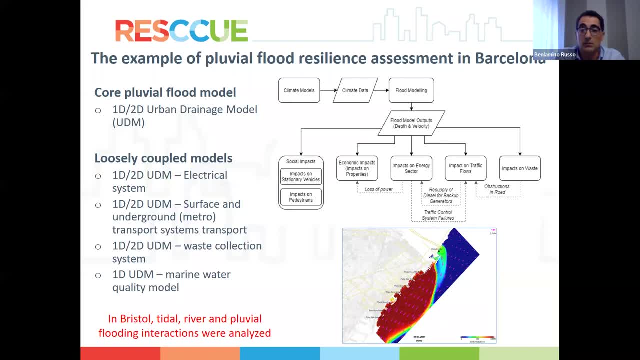 But also the impacts on vehicles. So the impacts, social impacts on vehicles- We assessed the possibility for a vehicle to be dragged by the flow And we also included economic impacts. So impacts on properties, on the assets of the city And, as said, on three main urban services. 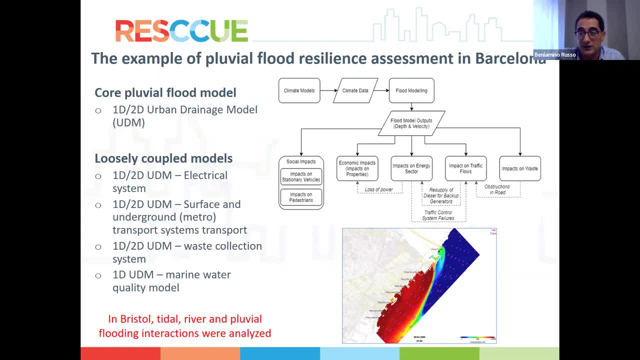 Electrical system, traffic transport system and also waste collection. From the results of this second layer of models, let's say we developed, we assessed cascading effects in terms of economic impacts due, for example, to increase of traveling times or a failure of electrical system. 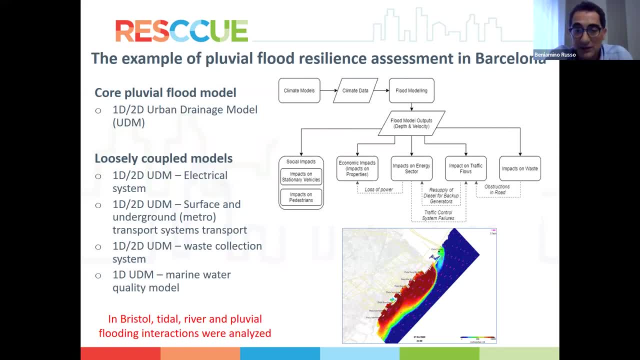 et cetera, And finally you are seeing at the bottom of the slide. we use also the outputs of the urban drainage system to analyze the water quality into the receiving water body, the Mediterranean Sea in Barcelona. Again, in this case we are looking at the contamination. 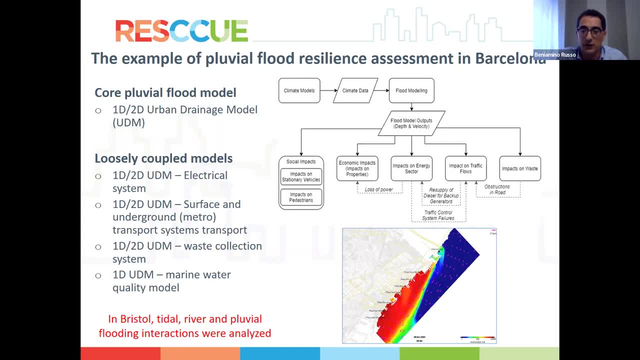 the pollutants produced by combined sewer overflow in the city, And here we analyzed all the impacts And we also analyzed also these data in terms of periods when the beach of Barcelona should remain closed, And these times, these periods, was traduced in loss. 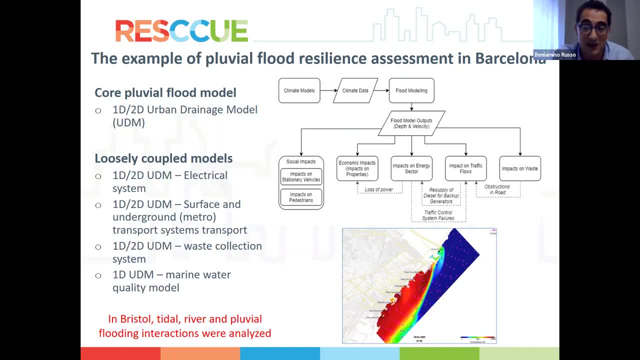 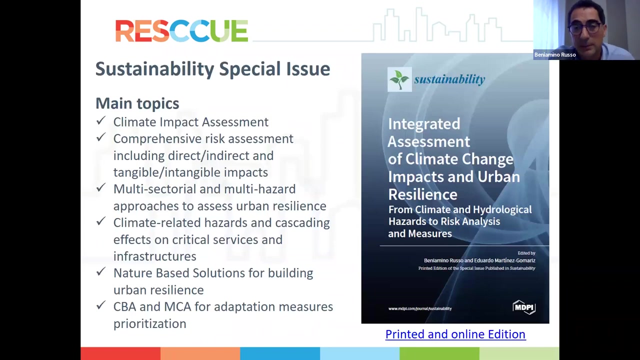 in terms of loss in monetary terms for the activities that are related to the beach. So we tried to analyze also these environmental and economical impacts due to the water quality deterioration produced by combined sewer overflow. I will explain part of the results, but if you are interested to have a deeper knowledge about the result of this project, 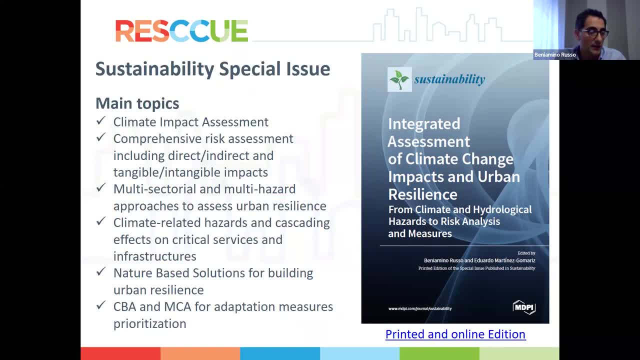 you could find more information in these special issues: Integrated Assessment of Climate Change Impacts and Urban Resilience. It was a special issue published as main outcome of the project. When you can find the methodology to analyze, to assess climate impacts on each one of these main services? 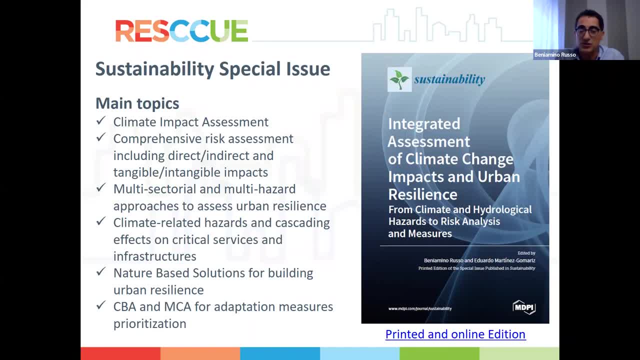 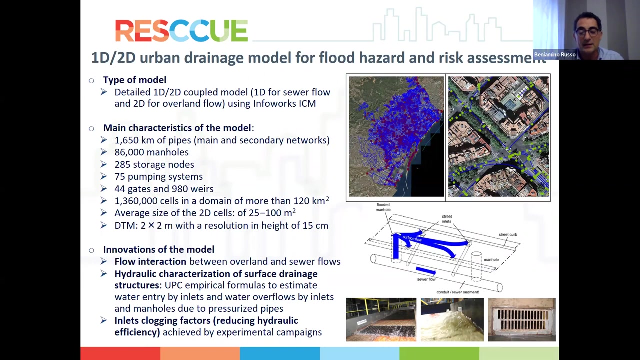 and also the effects of the adaptation measures that we propose to limit these impacts: cost-benefit analysis, multi-criteria analysis among different adaptation measures, method for the prioritization of these measures, etc. Okay, Moving to the main issue of this presentation, 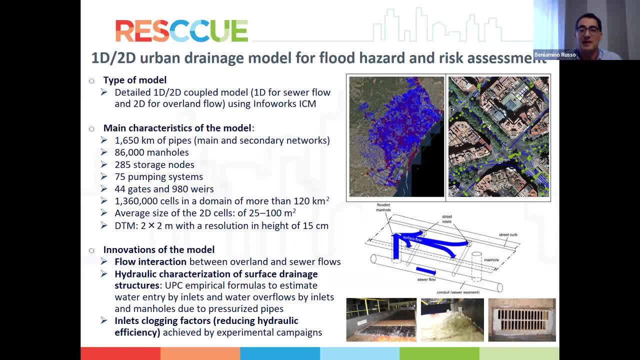 As said, we developed a very detailed 1D to D overland flow. We used Infowars, ICM. As said, the model covered all the city. We introduced main pipes, so main sewers, but also secondary pipes. We also introduced the concept of dual drainage. 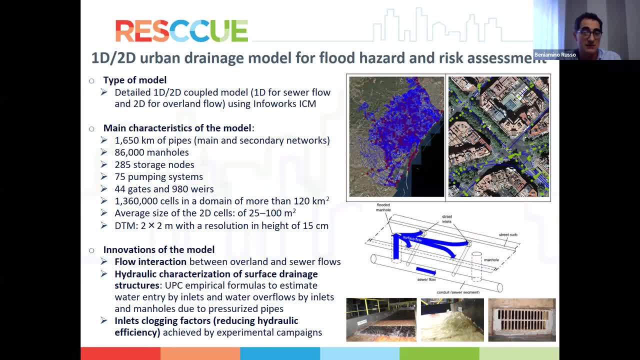 in the sense that we modeled the 1D sewer flow into the underground drainage network, but also its interaction with the 2D overland flow. The links between these two layers are represented by graded inlets and the manholes. We characterized these elements using experimental 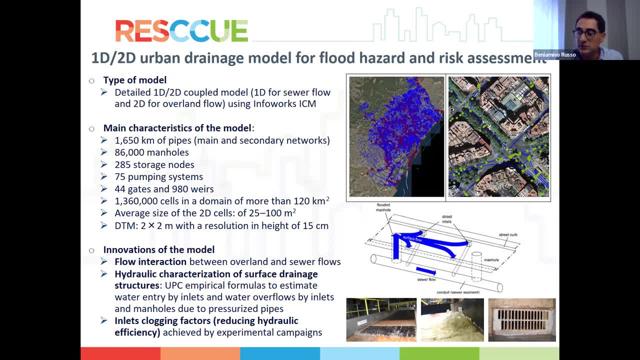 experimental equations developed at the Technical University of Catalonia in Barcelona, in Spain, that allowed us to characterize flow entry, but also the overflow in case of pressurized pipe conditions. We also introduced detailed digital terrain models, as you can see with a resolution of 15 centimeters. 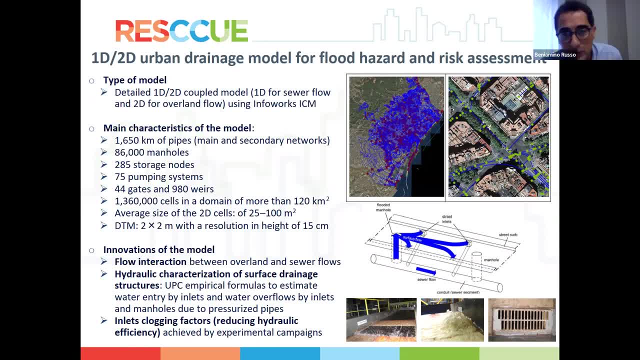 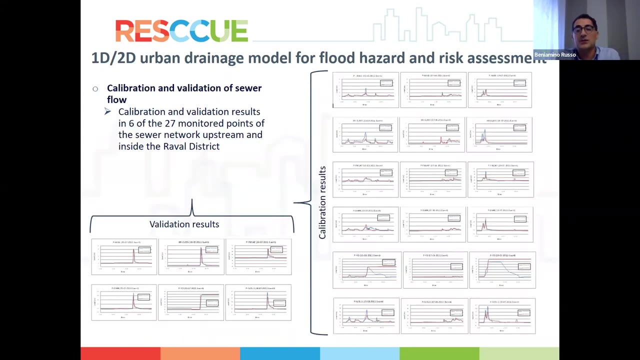 We introduced all the elements of a very complex- let's say very complex- network. so a lot of gates, a lot of storage tanks, for example, etc. This is the calibration: Calibration on the right, validation on the left. We used a lot of sensors. 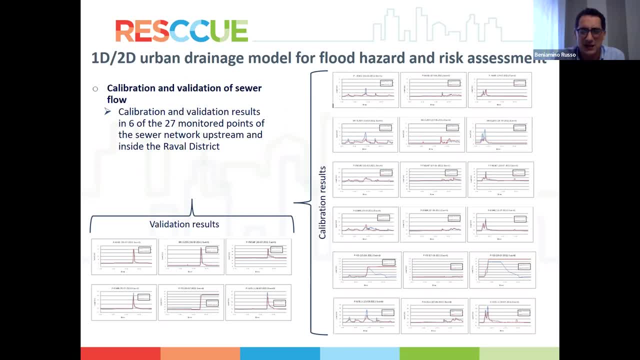 more than 20 rain gauge stations to calibrate the models and tens and tens of tens and tens of tens and tens of flow meters into the, into the drainage networks. So, as you can see, the calibration was, the calibration validation were quite good. 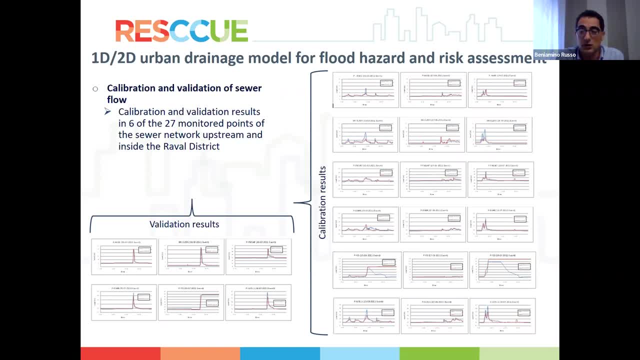 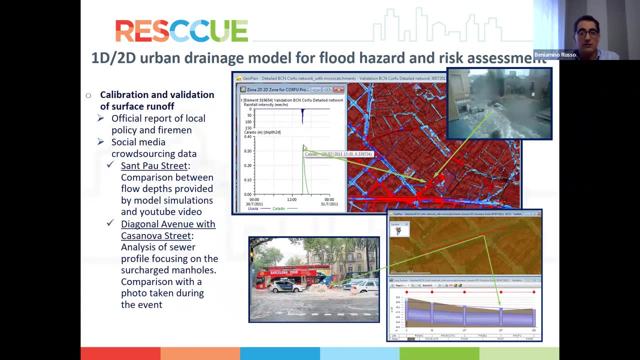 but it is solving the problems into the, into the network Outside. so for the 2D overland flow we used we used social media information in the sense that, for example, in this picture we are remarking. 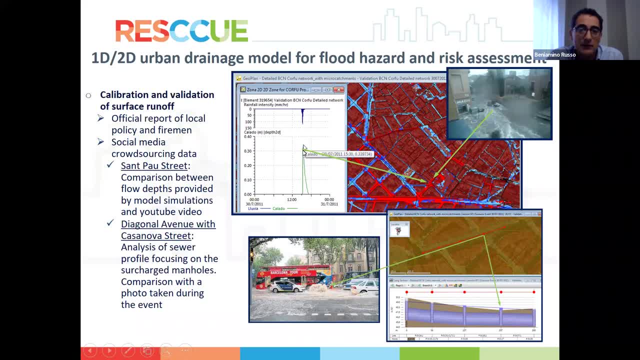 we are plotting the water depth in a specific cell of the 2D domain and these values, around 30 centimeters, correspond on the eight of the flow depth recorded by a video available in YouTube and recorded at the same time of this. 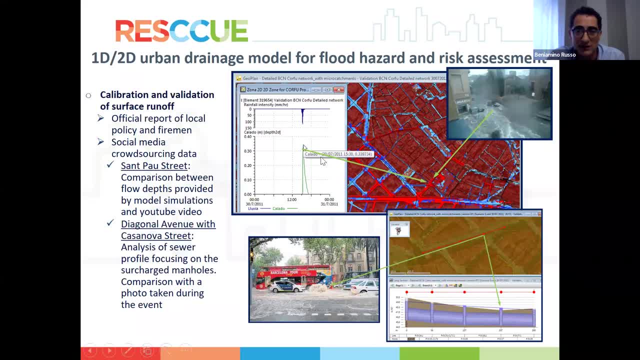 events used for the calibration occurred at the end of July of 2011.. Another example: this is the a cross, a crossroad between Diagonal Avenue and another important street of the city, As you can see here. 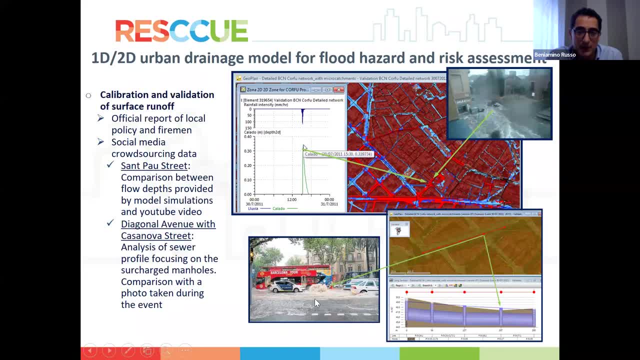 we have pressurized pipes with piezometric, with an overflow and the piezometric level that reach the eight of, let's say, one meters maybe above the, above the, the terrain, In this case. 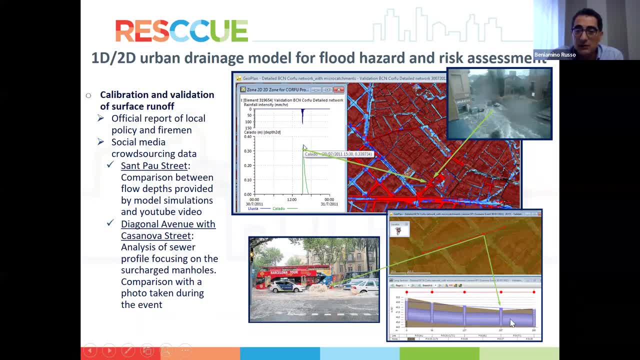 we are validating the 1D, 2D models using this kind of data. So reports from the police, firemen, YouTube videos, photos et cetera. Okay, when we developed 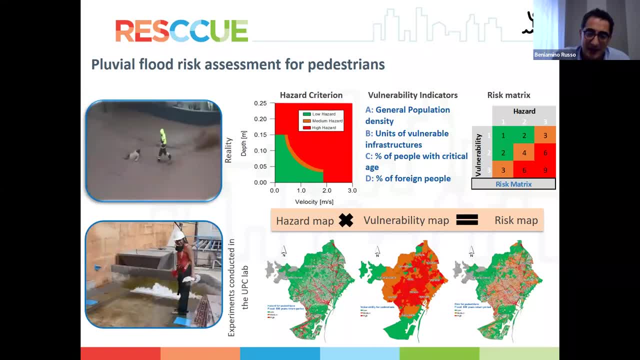 the models. when we calibrated and validated the model, we used this model to assess risk for, I say, pedestrians and also vehicles. One of the innovation of the project was the use of 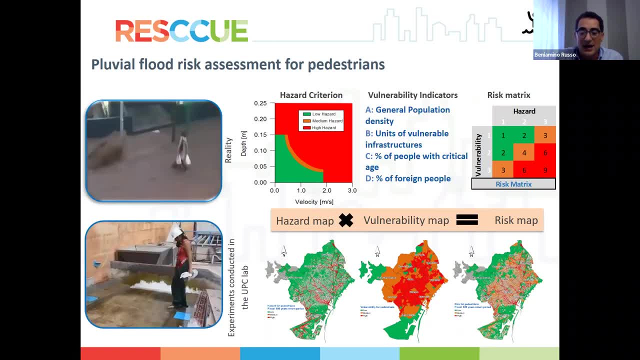 specific hazard and the risk criteria depending on the risk receptor. It's clear that we cannot use the same hazard thresholds for people, for vehicles or for waste containers, for example, in case we want to. 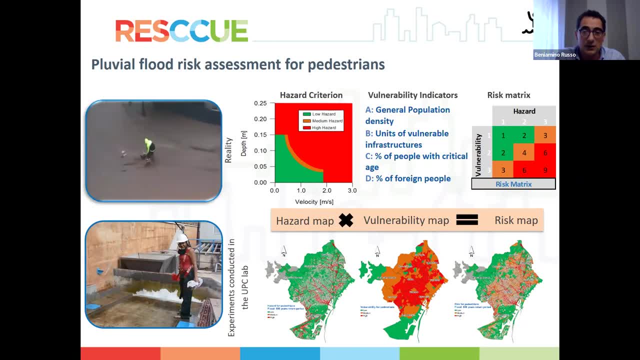 to know where they are dragged away. So in this case you are. you are seeing the specific hazard criteria developed, achieved again, trial experiments conducted in at the hydraulic laboratory of the 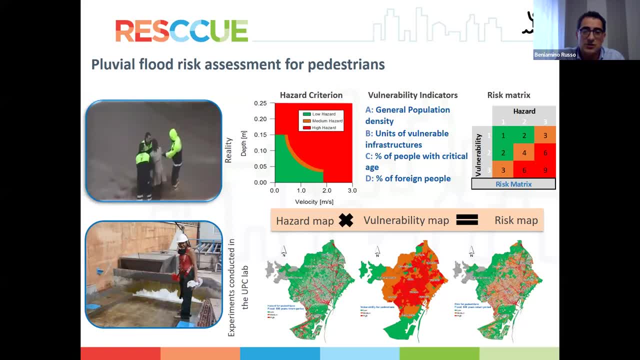 of the UPC Technical University of Catalonia that show that a palm of water- so more or less 15,, 20 centimeters, as you can see in the first video- can drag a people. 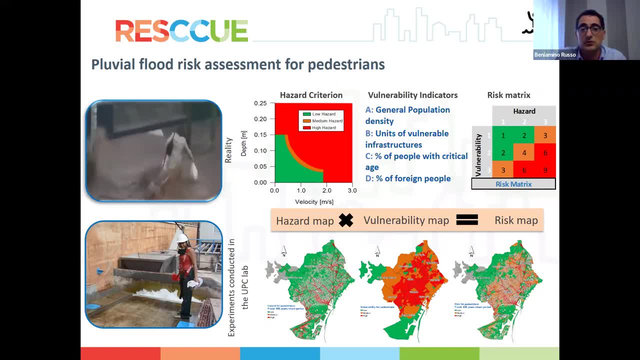 when the flow occur with the velocity of two, three meters per second. Generally, the other criteria used in bibliography are more related to river floods. So the typical condition river floods is to have. 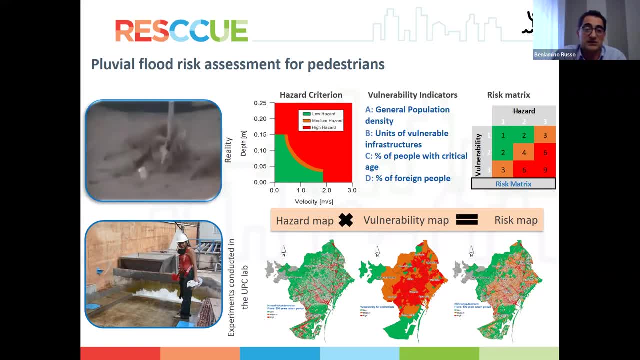 one meter of flow and velocity, reduced to one, two meters per second. As you can see, a palm of a palm of that 10,, 15 centimeters linked to a velocity. 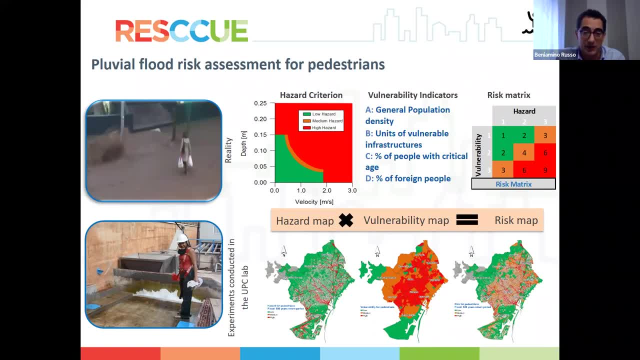 of two, three meters per second are able to drag a person. So to suppose hazard for a high hazard for for pedestrian that are crossing this street. We so, we demonstrated. 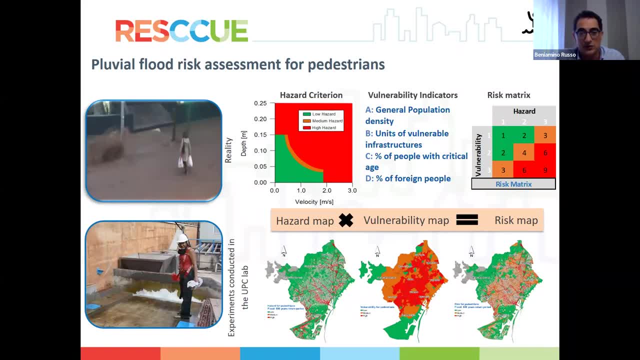 with test, hundreds and hundreds of tests of specific flood hazard criteria to be used for pedestrian that can cross a flooded street during this kind of events. Then we cross these hazard maps. 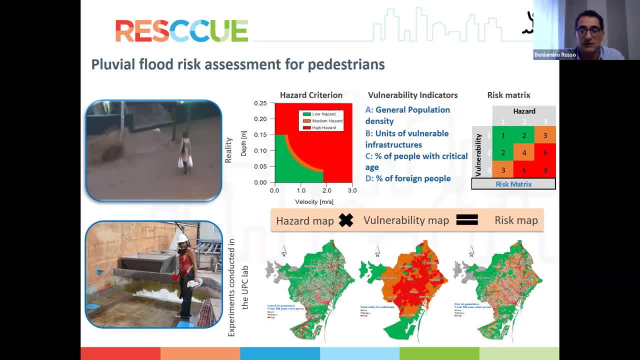 computed, developed using these hazard criteria, with vulnerability maps based on indicators like population density, the presence of vulnerable infrastructure, other school or hospitals, the percentage of people with critical age and percentage. 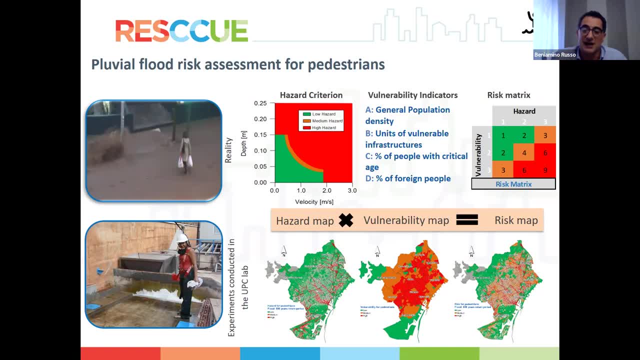 of people, of foreign people that could not understand the alert and the message for evacuation, et cetera. These indicators were used also in other European projects, like flood site projects And then. 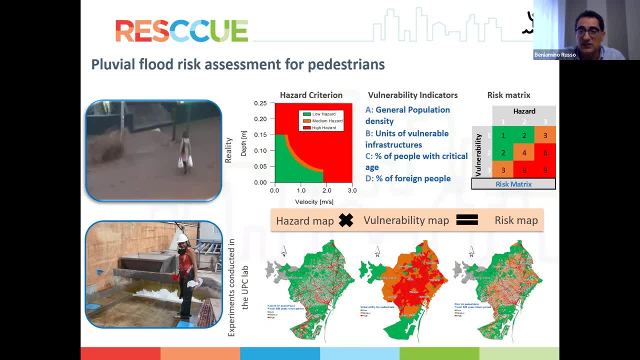 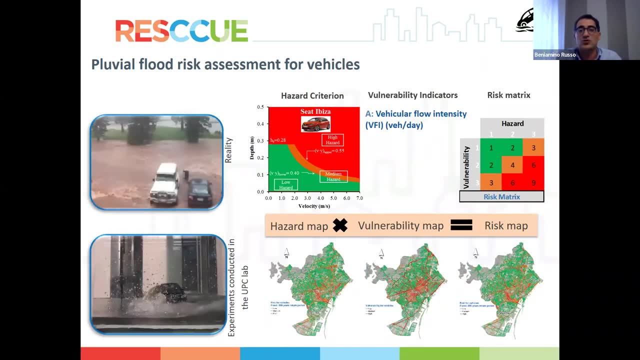 finally, we produced a qualitative risk map using a classical risk metrics. As said, we have to change the hazard criteria when we change risk receptor, So in this case we used again other 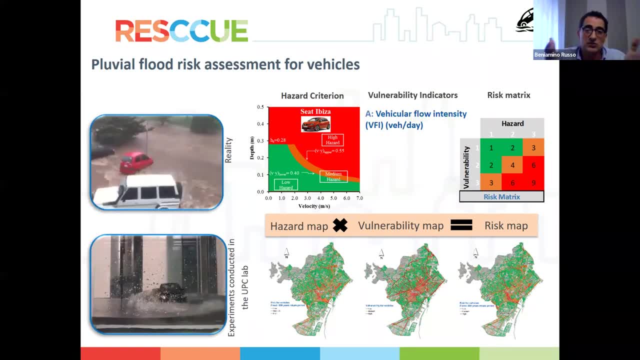 hazard criteria related to the most common vehicles that we have in Spain. the SEAT Ibiza is a and, of course, we have a critical flow depth at which the, the, the 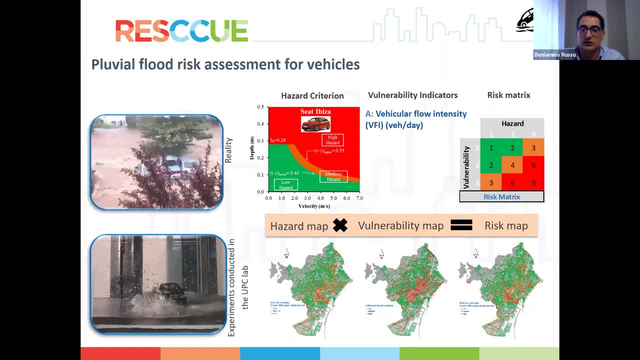 the the vehicles could loss could the losses is it's instability due to the float: flotation but so our sense of velocity. but when we have a flow with two, 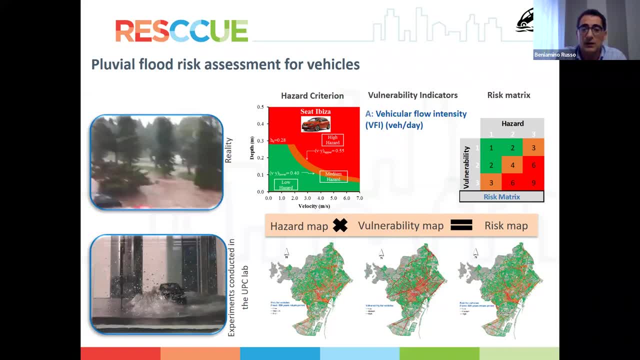 three meters per second, again we could have the situation, the same situation, a similar situation, respect to the pedestrian one, so we could have instability or this dragging phenomenon for water depth. 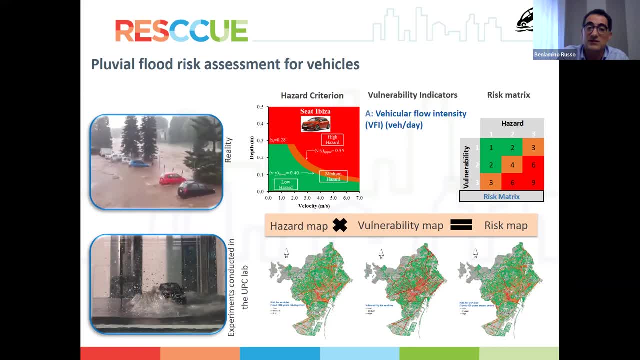 around 10,, 15,, 20, centimeters for for for this kind of vehicles. so we changed fluid hazard criteria for this new risk receptor, in this case vehicles we produced. 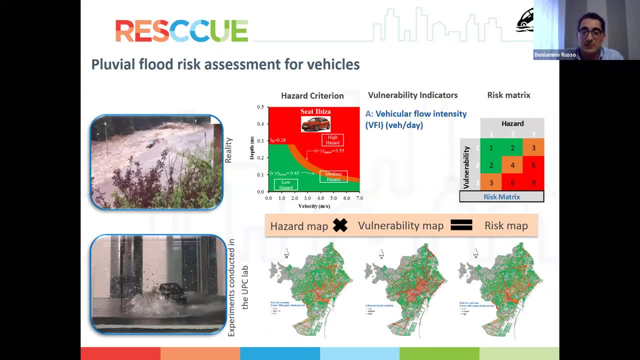 new hazard maps. we crossed these hazard maps with, in this case, simpler vulnerability maps, only based on on the exposure, on the vehicular flow intensity. in the other case, we used also the. 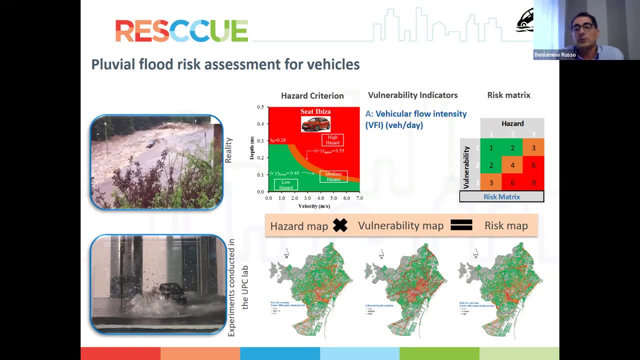 intrinsic characteristic of the risk receptor. and we performed again a risk, a qualitative risk assessment, using again a classical risk matrix and achieving risk maps for several return periods, several. 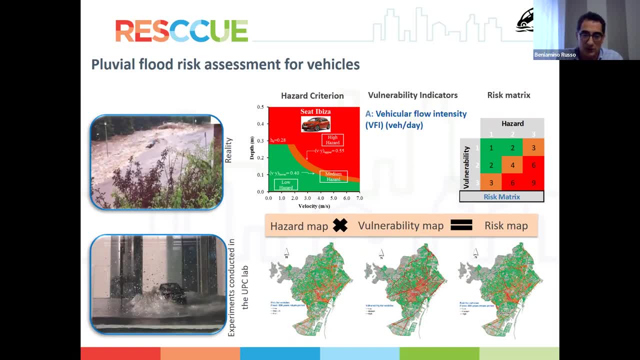 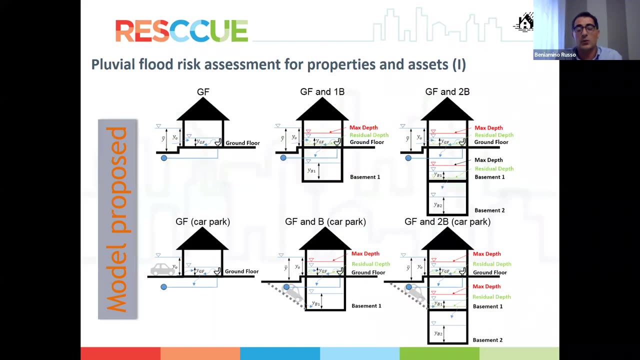 climate change scenarios and, of course, also the current situation and future situation, considering business, social scenario or adaptations scenarios. we also developed, I said, all this information, all the papers. 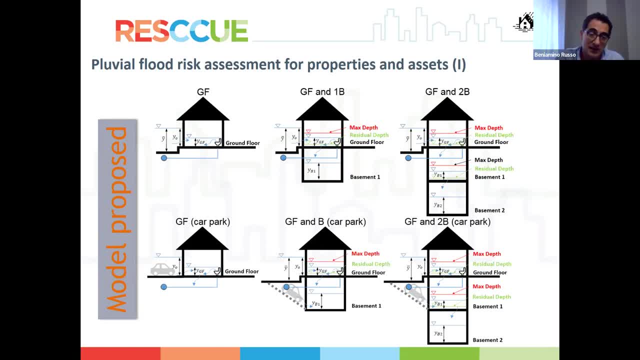 related to these methodologies have been published and included in these special issues that I have presented before. about the economic assessment, we propose a model that demonstrates that type of 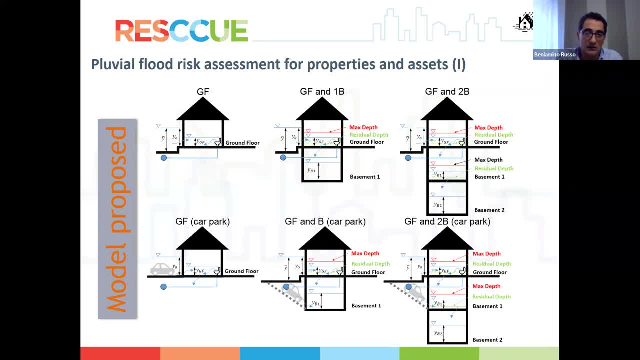 of buildings. so in this case you can see the first case of of a building with only the ground floor. then we have a ground floor at the basement, ground floor into basement, et cetera. 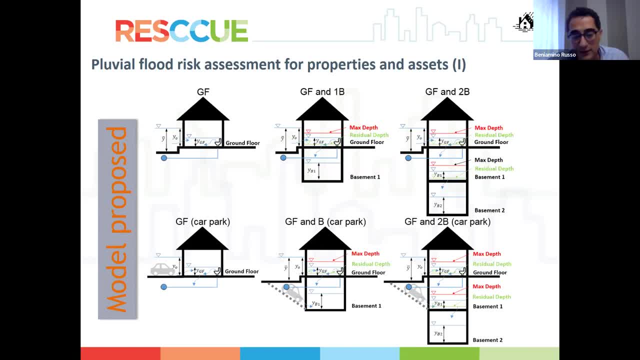 so the idea was to to to find the core, the, the relation between the flow that outside, inside the building. for this relation we use an experimental data and also. 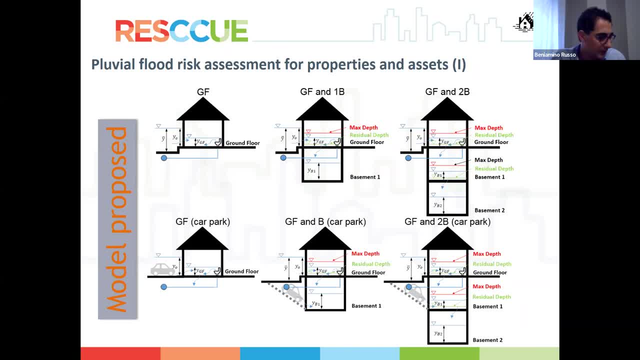 opinion of the insurance experts that worked in this, in these fields. we contracted several studies in and we collected a lot of data. then we the the Spanish minister that 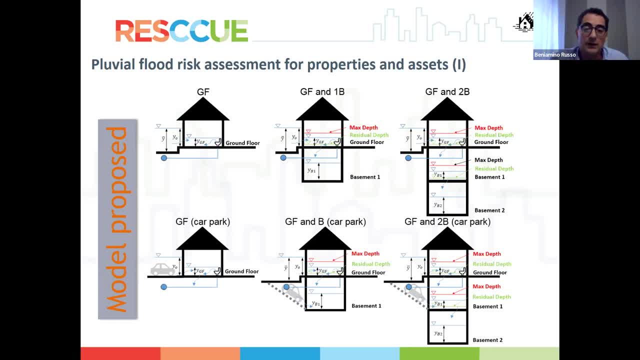 managed an entity for for for for disaster, provided us historical data for each parcel of the municipality, with the location, with the claimant, with the claims, with insurance. 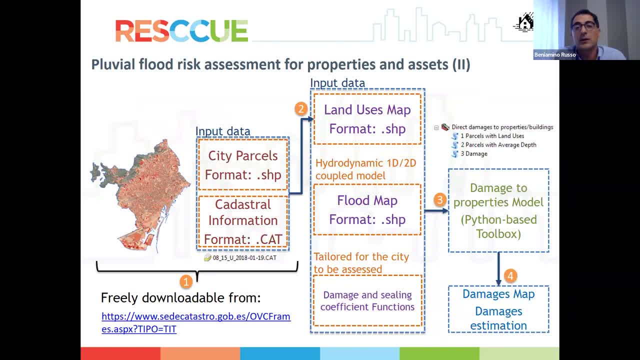 cover, et cetera. and finally, we develop it a a tools that use the city parcels, information that could be downloaded, downloaded, at least in Spain, from the 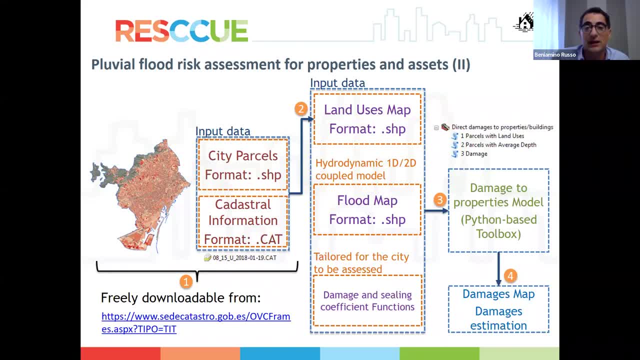 cadastral entity and on the basis on land use map for each of the floor that we are analyzing. provide a damage a provide damage information, of course also. 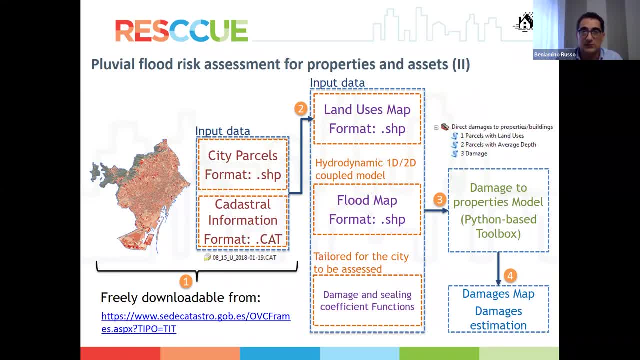 using the outputs of the aerodynamic models in terms of 1D- sorry, in terms of flow depth information and, of course, we also use it. we produce. 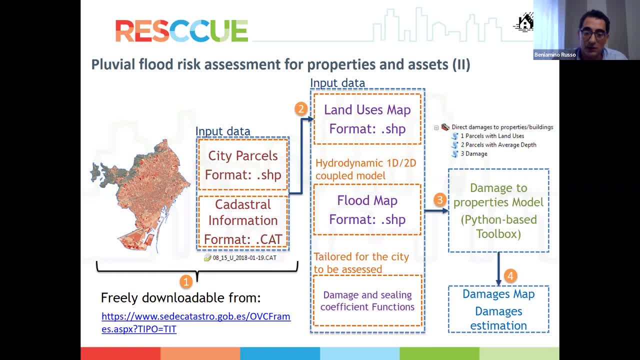 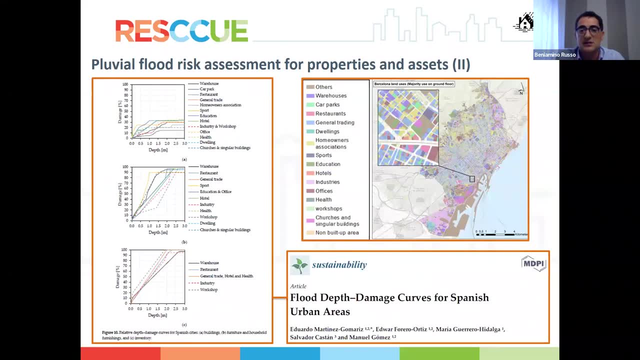 it to link the flow depth outside the building with the flow depth inside the buildings. again, this information has been published and is available in. 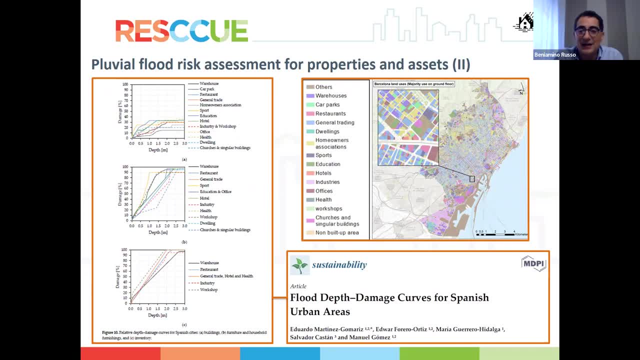 these special issues as set of land use, we 14, or 15, land use to be used, because I said we perform this, perform this. 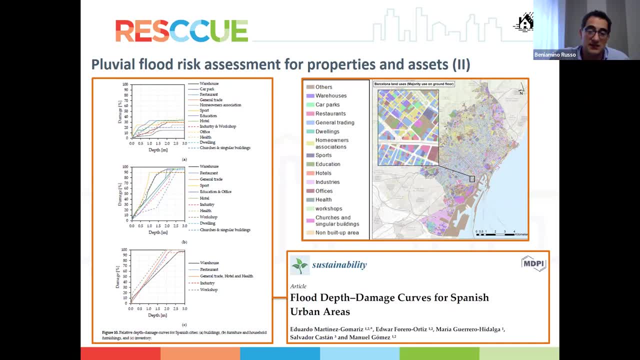 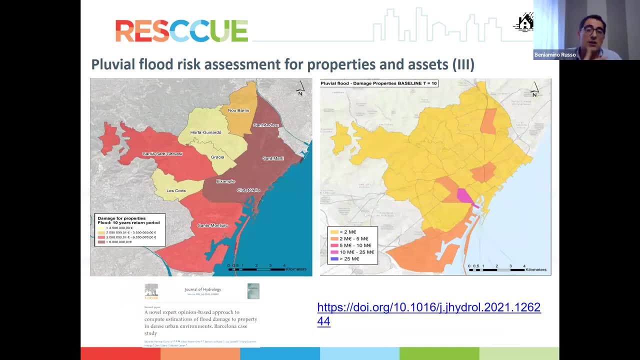 analysis in all the city of Barcelona, with these tools and all these knowledge allowed us to create these risk maps, these times in terms of 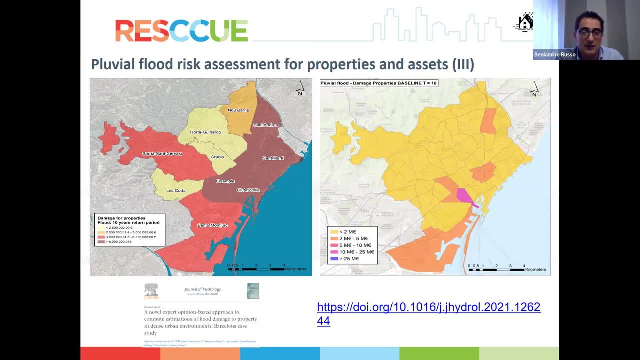 tangible damage. so economic risk assessment. we produced these maps in aggregate just to avoid problems with with the data, but originally we add the data. 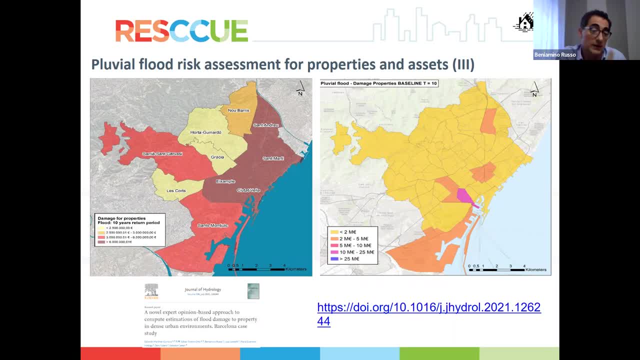 for each parcel, but we decided to present, agreed with Barcelona municipality, this, this information for the case. the tools and the meters were published on. 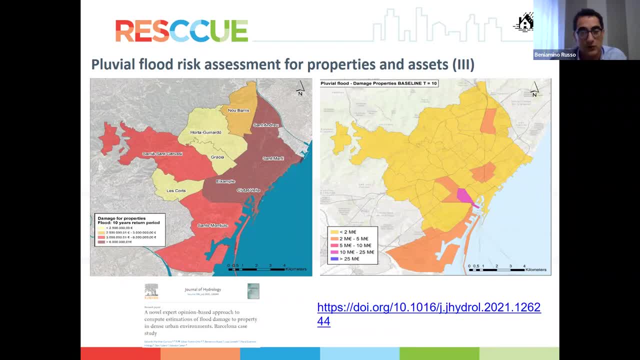 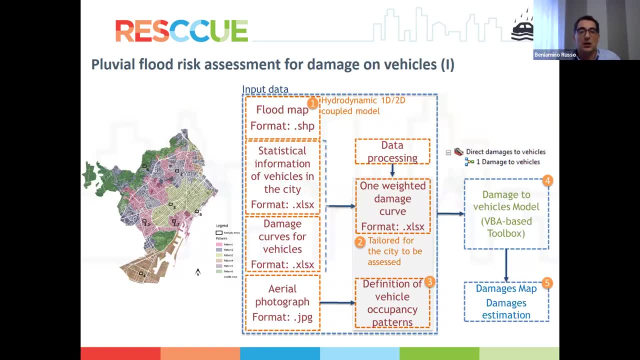 on on another journal, journal of hydrology. here you have, you have the doy and the title of the we had. we found that around 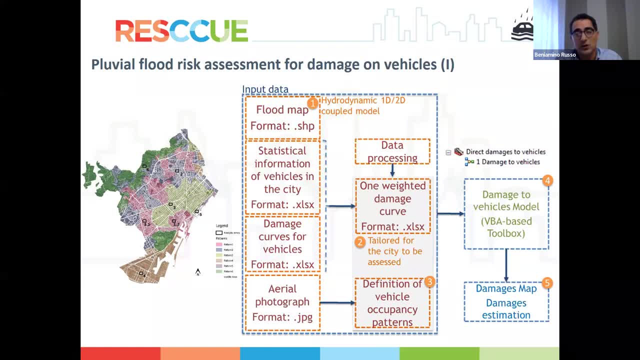 10, 50% of the total damage occurred during flooding events could be related to to the vehicles, so we developed and similar approach in density. 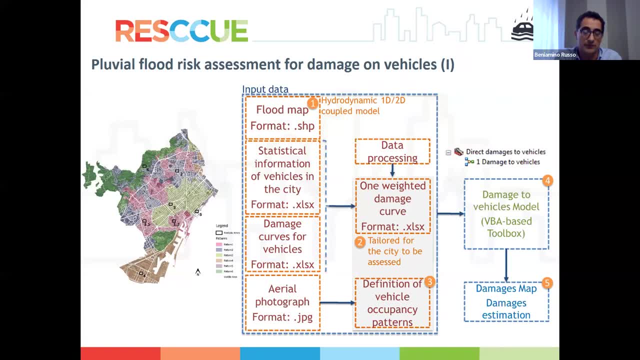 a potential density of, of, of the of the vehicles, of the vehicles in each district, street, et cetera, and we use, in this case, 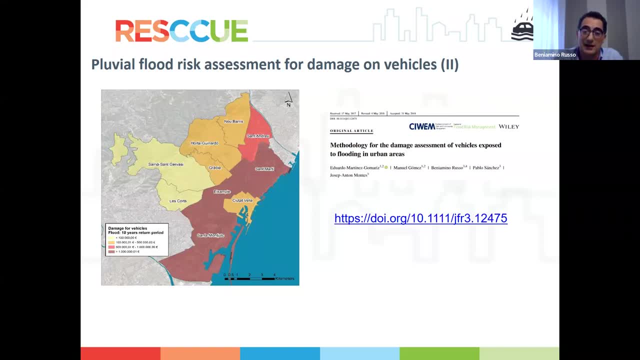 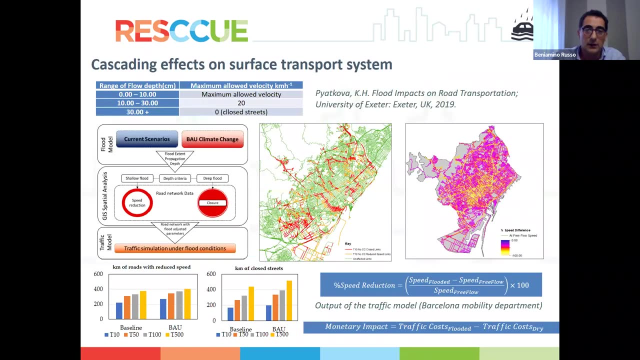 existing through them, through the economic risk related to damage on vehicles, about cascading effects on surface transport system. in this case, we worked with 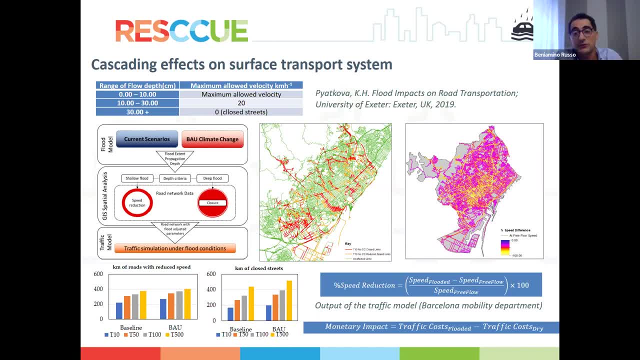 Exeter University. they are a specialist in this kind of the outputs. first of all, we have these rules in case of having a a 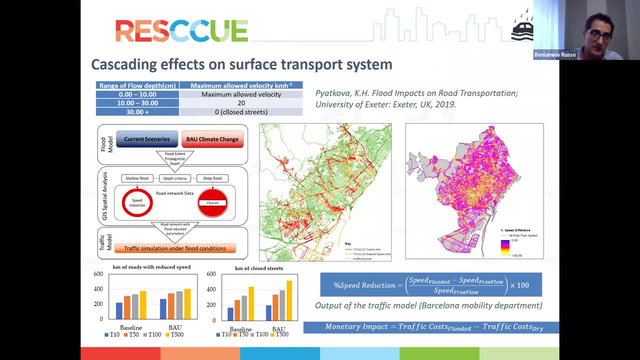 flow depth from zero to 10, centimeters. we could consider that the maximum velocities. for more than 30, centimeters, we considered the streets as 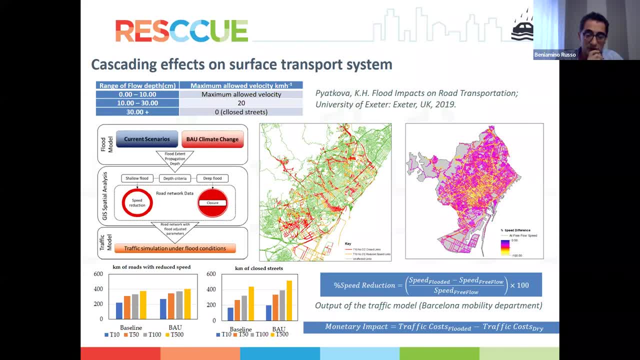 closer. okay, so flow depth. this flow depth output from 1d to d drainage models. this kind of information allowed to calculate the speed reduction. 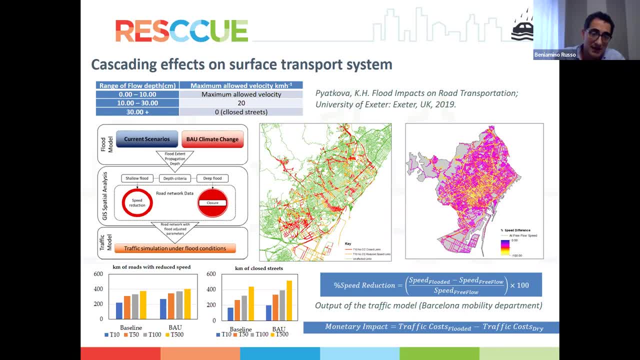 in the streets, in each street, for several again, for several return periods, for several scenarios again: current state, business, unusual and adaptation scenarios and speed. 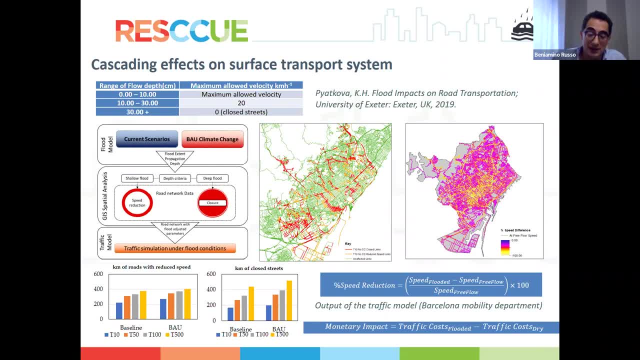 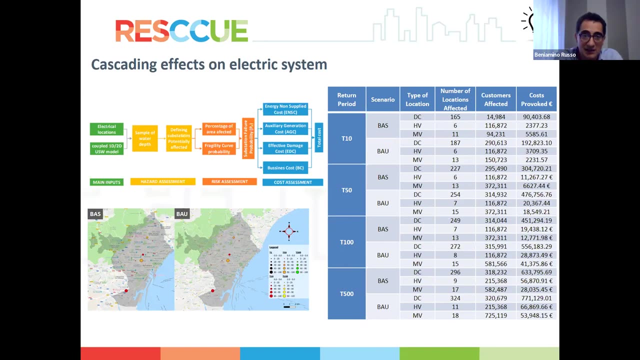 reduction, the, but also environmental impacts like the increase of fuel consumption, et cetera, for the cascading effects on an electric system. you can see: 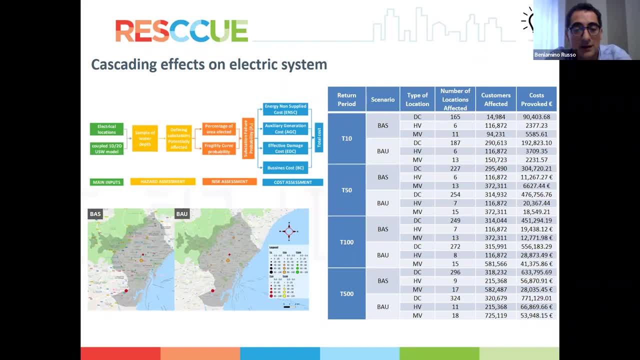 again the scheme we the typology of of the electrical infrastructure. on the other side we add the wanted to the outputs, just to remark. 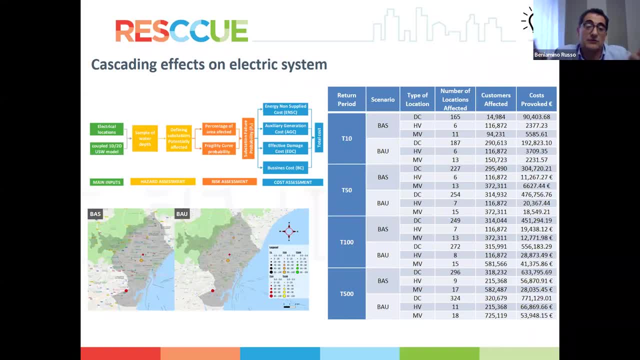 we, you said, always flow depth in this in case- fragility curves for substation or distribution center, et cetera- in order to reach the 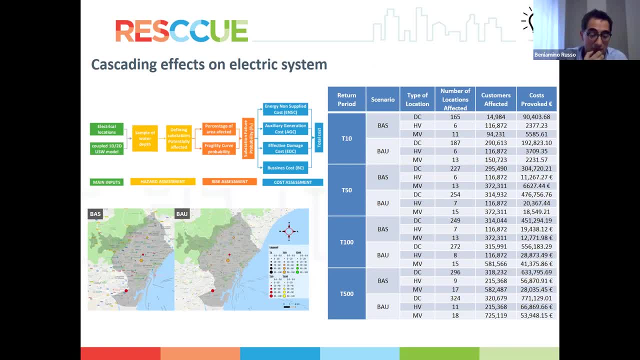 failure or not of this kind of infrastructure and this kind in case of of that, of course, one of the of the partner in our 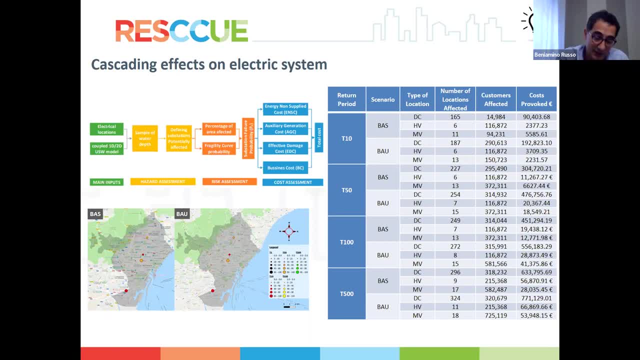 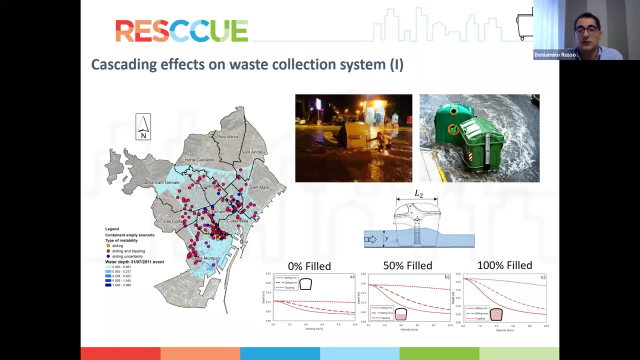 consortium was the company to manage the electrical system in this in the city, and also the techno, the analysis of the stability of waste containers. 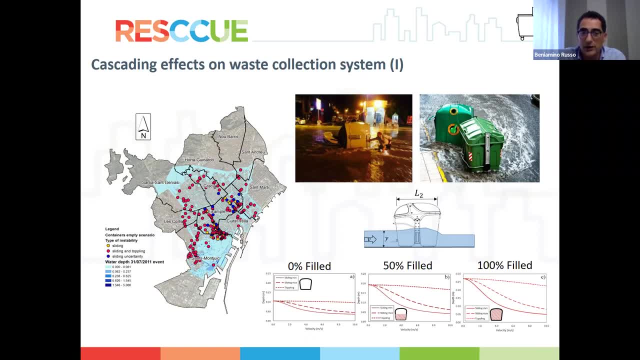 into the city, depending on the percentage of filling of each of these containers, and we analyzed the potential stability of these elements of mobility sliding. 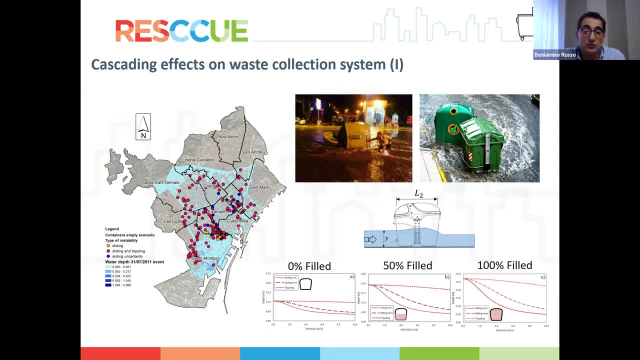 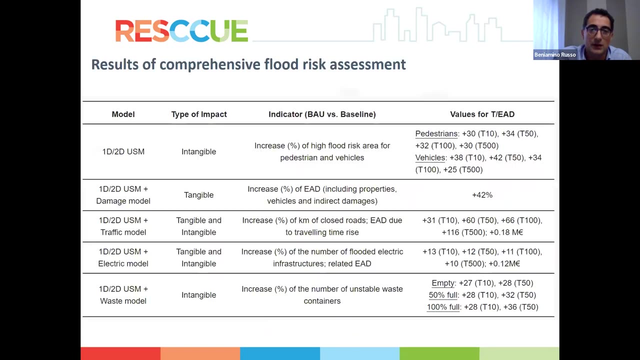 toppling, et cetera. We also tried to validate these, these models, using again reports, videos occurring during real events And, finally, as results we could. 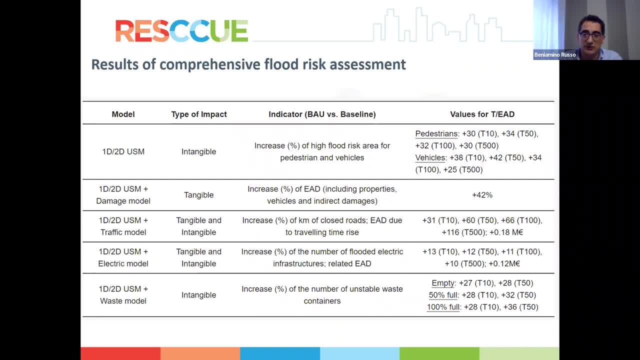 provide, let's say, for the risk assessment in terms of intangible damage, like, for example, the high risk area for pedestrian, for vehicles, in terms 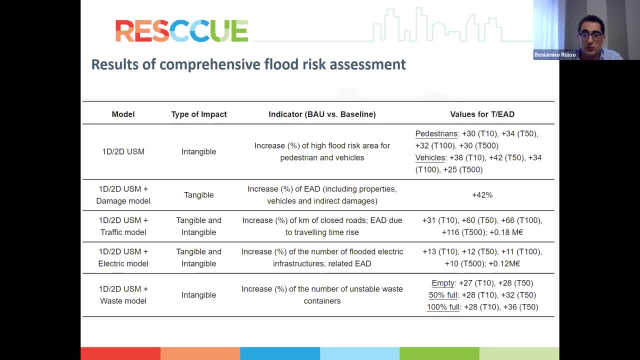 of increase of this area for the future in damage the. there is another publication about about that. but all this information where this was expressed, 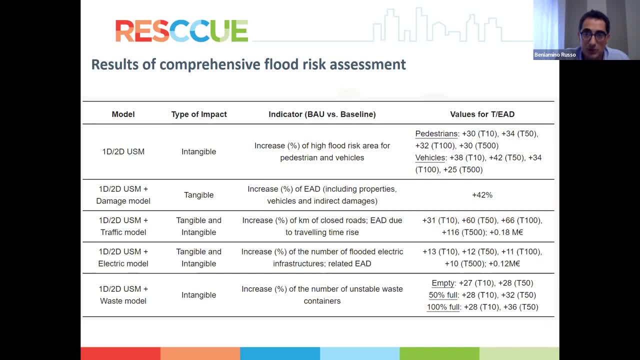 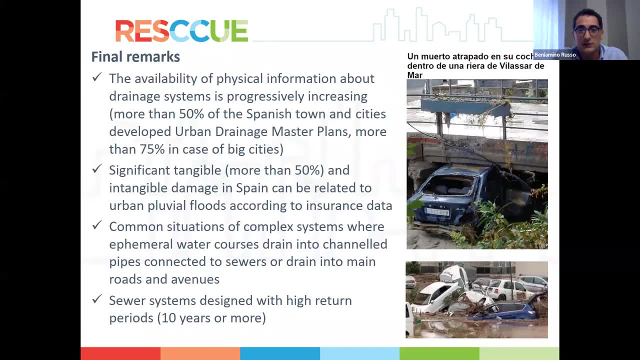 in terms of expected damage, and this in this expected damage, for example, we considered that the lack of information, of physical information, topographic information, 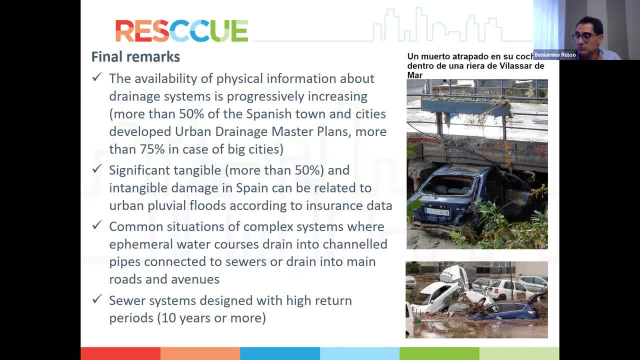 about urban drainage system, supposed their um neglection in the assessment of of flooding, for example in severe floods and pluvial floods in urban. 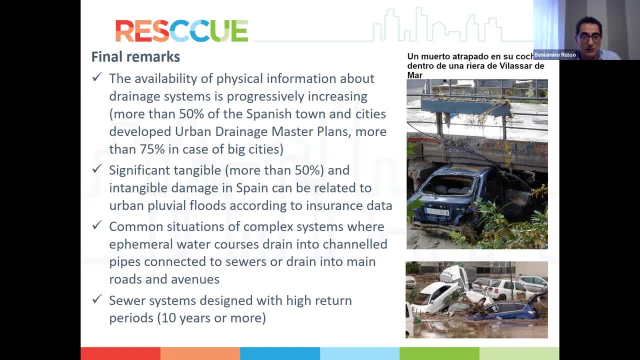 areas, and the reason was, of course, related to competence, but but also related to, to the, to the lack of data in the case of 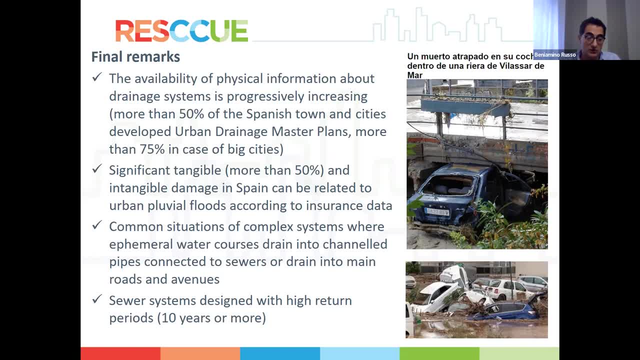 big city, as demonstrated also by the claims of this historical data that we used the the. the damage produced in urban areas by pluvial 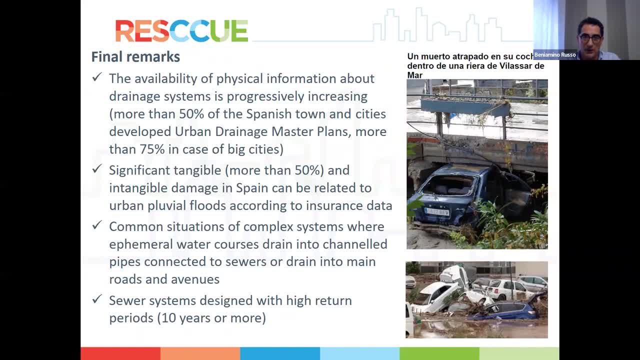 floods. mainly due to flooding, many times, at least in the south of Europe, it's quite difficult to distinguish between ephemeral water cores that there 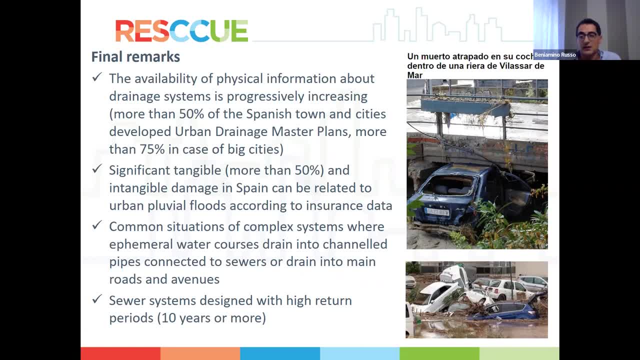 are channeled in pipes with respect to life lived together in our urban environments. another remark is about the return period in the south of 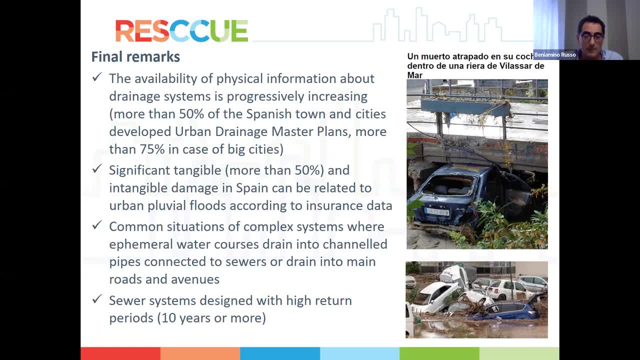 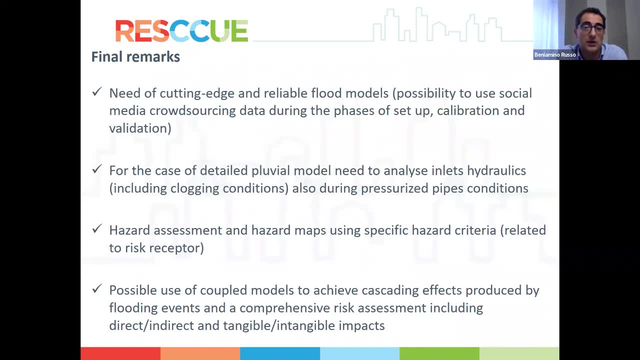 Europe and in Spain, for example, the classical return period values used- let's say innovation in terms of methodologies, tools and impact models- to perform. 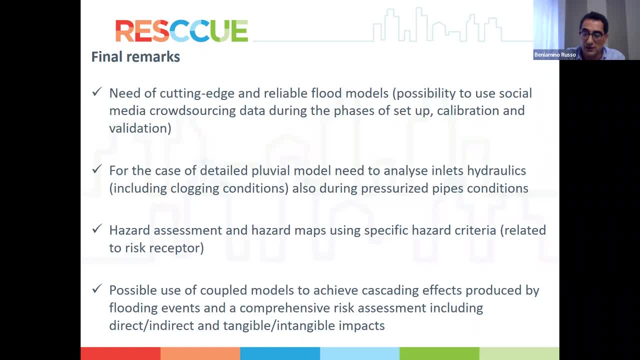 this kind of analysis. we were invited to directive through directive working group to explain some of that we- that I personally did- is to use 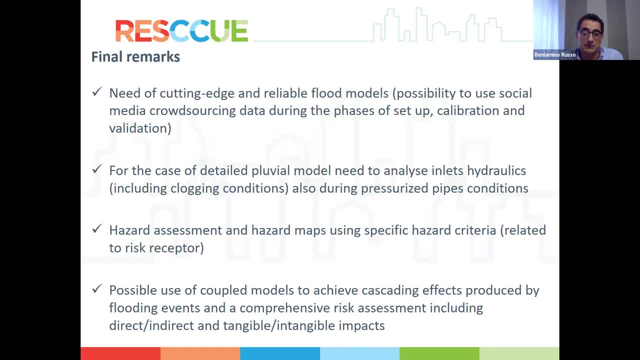 specific hazard criterion. specific risk criteria depending on on the risk receptor is not current to have one hazard maps or complete models to be calibrated. 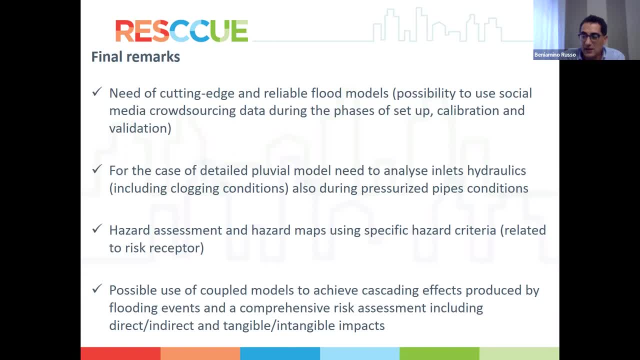 to be validated using the dual drainage approach, the elements of the greater village to be characterized, et cetera. of course, we have to use 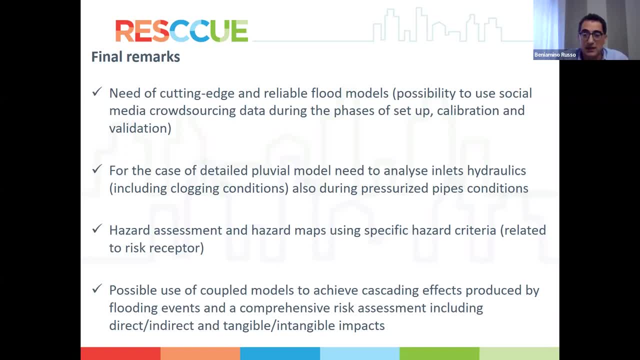 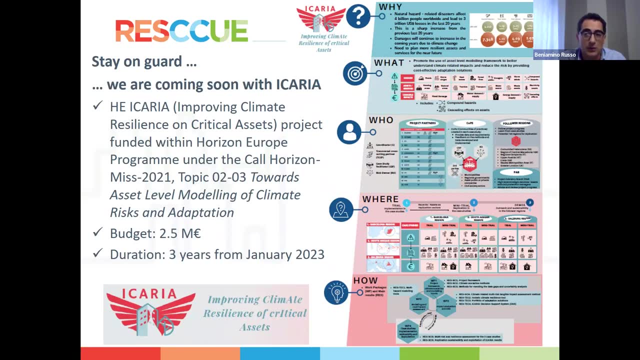 and to help the decision makers. I think that we could use them and just to inform you that Aquatec- we will lead another project. 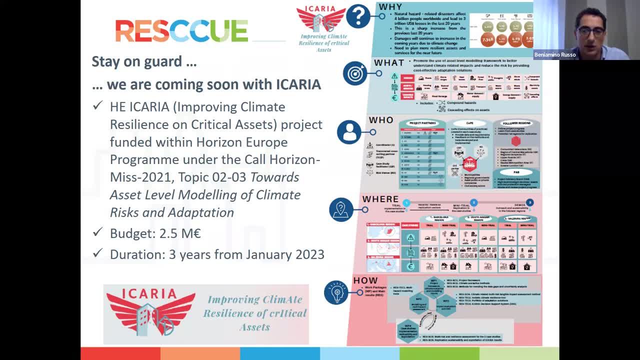 in this. in this project that will start in January 2023, we have again three cases study, this time all the Barcelona metropolitan area and 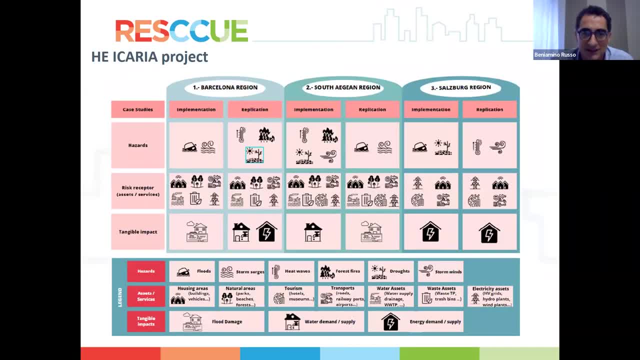 we have again three cases study, this time all the also Salzburg region in Austria and in Greek, as you can see at the bottom. 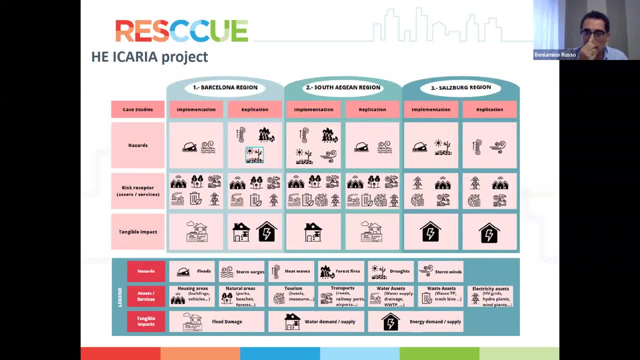 of the picture. again, we will analyze several climate related hazards and again the natural area. so rain infrastructure will be considered the same both as 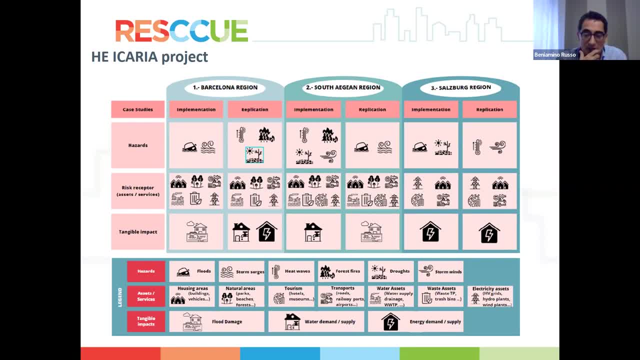 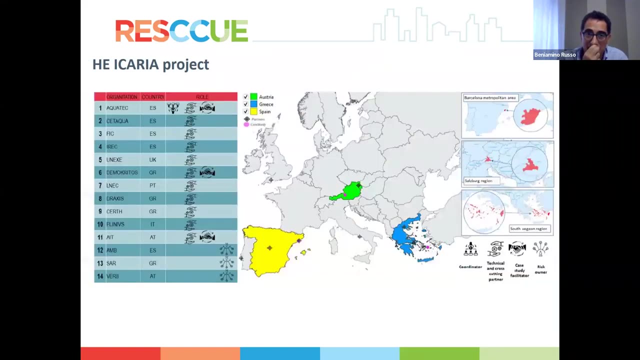 risk receptor, so as an important infrastructure or critical service to be to be impacted by by the, the risks and the the the change and. 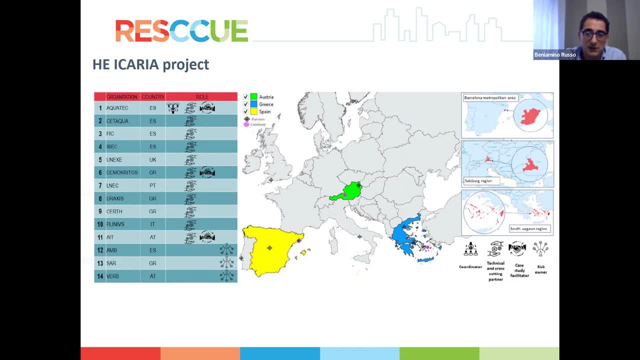 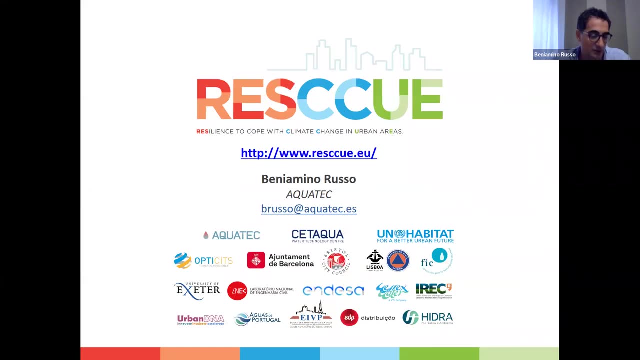 the, the, the, the, the impact or change or change of of of human fish or humans, or to explain or to clarify any doubt that you can have. Thank you. 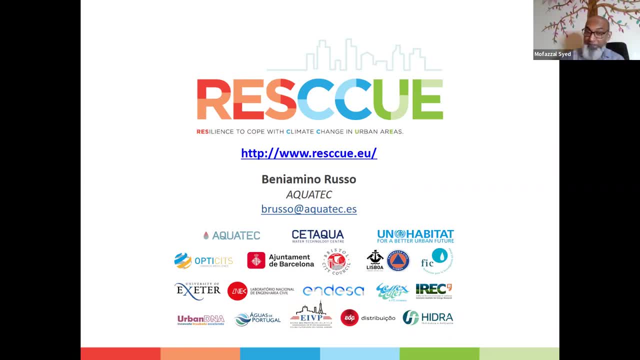 Thank you, Professor Russo. That was very good presentation. We did a lot of analysis and I didn't know that you could collect data and dynamically linking those utility services and transport maps, which is very good to know. Please give any questions you have in the Q&A boxes. 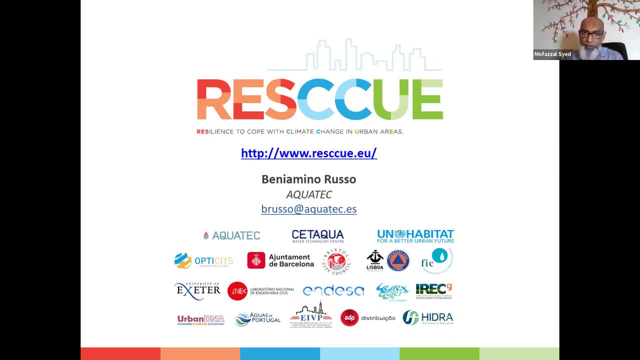 while we are waiting for some questions, I have one question, Professor: What level of satisfaction did you receive from those three cities that you have applied, from the local councils or the administrative bodies? First of all, we have to remark that we selected these cities. 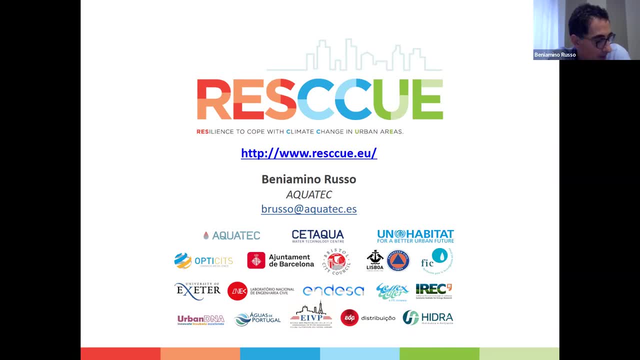 because they had a city resilient officer, so a coordinator, a key player in the world of the resilience. So these cities had a passion for the city and they had a pathway, a previous pathway, previous to the rescue project, And so the work during the project was easy in the sense. 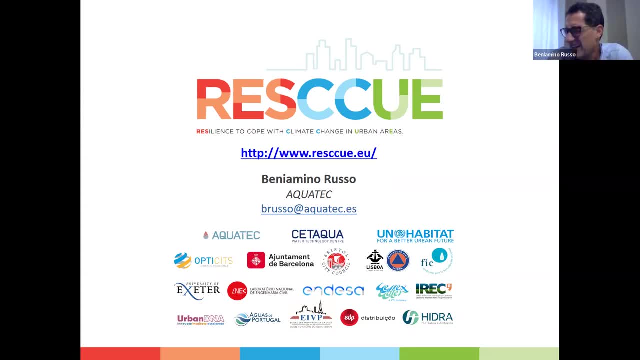 that we had clear the operators, the people to provide information, the requirements, etc. In these terms, the degree of satisfaction was, I think was, quite high. Thank you, Thank you, quite high. For example, we developed a resilient action plan including all this information. 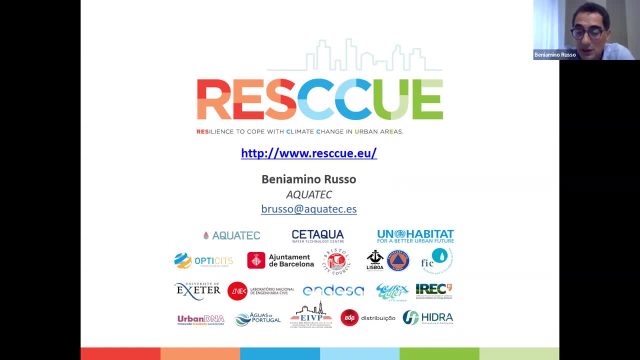 and helping to define or to stress the needs of some adaptation measures. As we have seen, climate change impacts could increase economic and social risk of around 30,, 40, 50% respect to the current situation. In the case of Barcelona, the results were also used and included in. 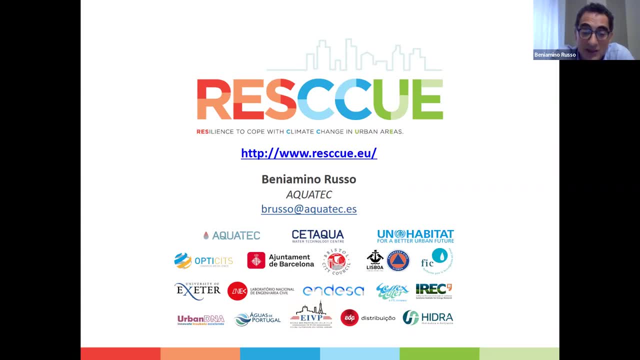 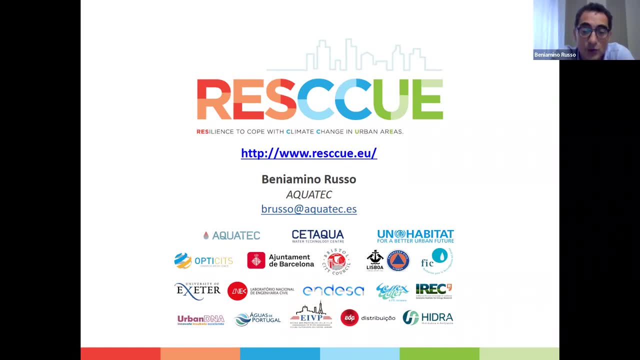 technologies- the models, of course- was used for a practical use and will serve to justify investment of millions and millions of euros. So I think that it's a clear response to your question. Okay, And you mentioned in one slide that in South of Europe you prescribed more than. 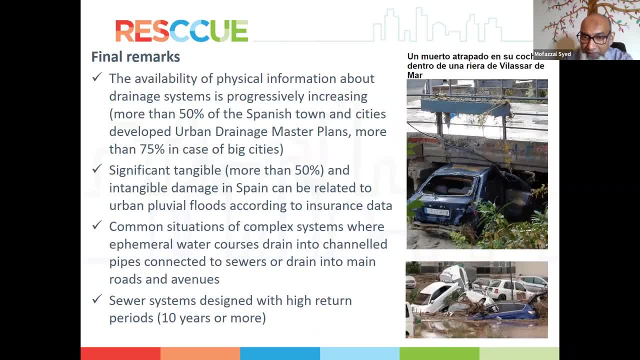 10 years design, 10 years return period design, Whereas in UK this is 30 year plus climate change. So in Bristol did you use this 30 year plus climate change standard for Bristol study? No, it's true that, at least during the last years, the standard return period criteria 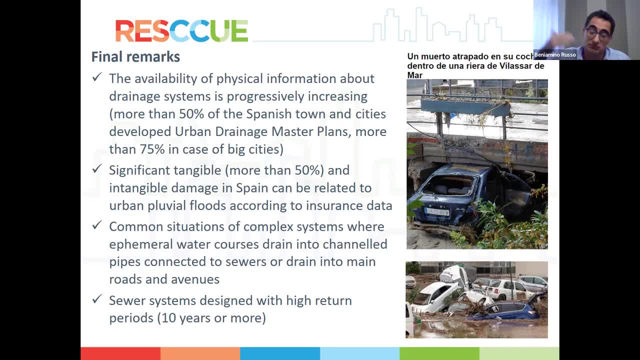 have increased in the North of Europe after several decades that were more close to five, seven, et cetera. In Bristol, it's true we used more restrictive return period, around 20 or 30 years, but we have to consider that all the existing infrastructure was designed. 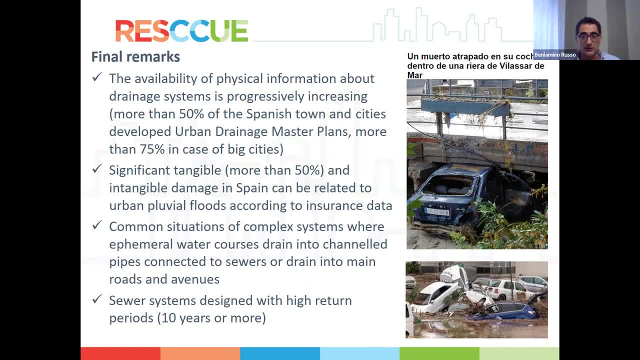 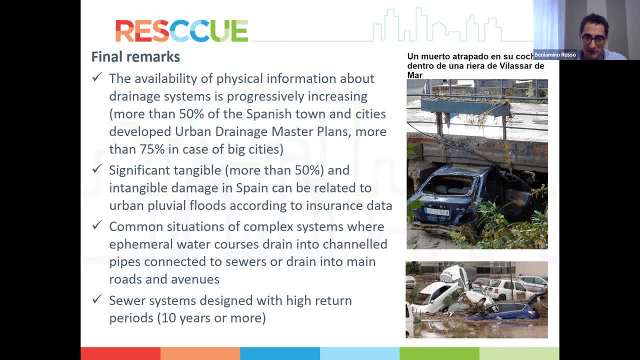 dû duaverage remind those of early. And of course these return period are related to future rain falls, the in-break waves, future design rainfall. So let's say we are applying this return period to maybe increased yetto graph due to the climate change factor that we generally apply to take into 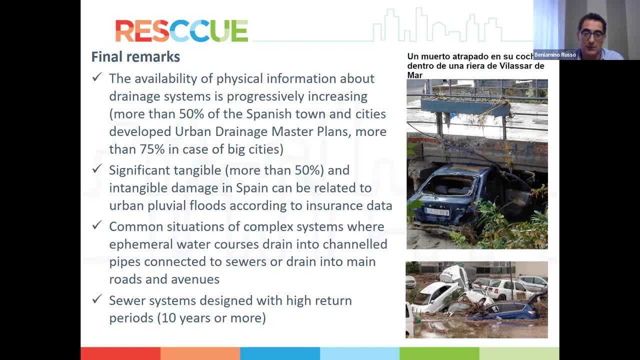 account climate change effects on maximum rainfall intensity. So what sort of climate change uplift do you do? What percentage? We developed three different studies of local. We need to perform local study to achieve these factors. In 2015, we used a climate change factor of around 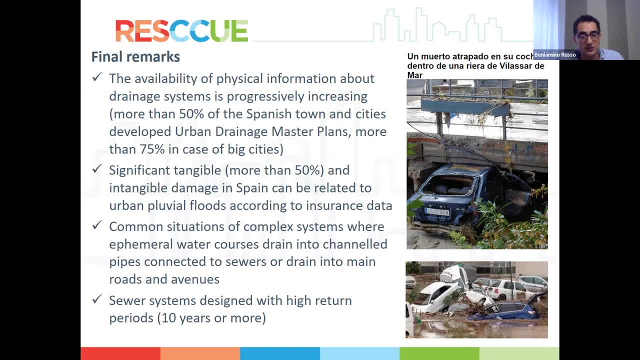 12 percent for all the blocks of the yetto graph. In the rescue project we achieved climate change factor for each block and each duration of the rainfall, But the climate change was ranged from 10 percent and 50 percent, And in Madrid we found more or less similar values around from seven to nine percent. 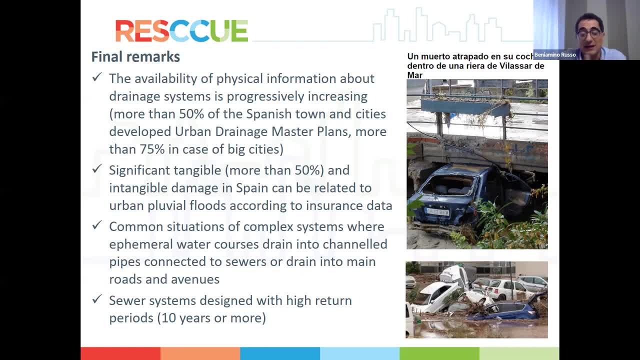 It's around 10-15 percent. the result that the climate change factor that are currently used in Spain for a return period of 10 years. Okay, okay, thank you very much, And we've got a question from Roger Swan. He's into specifics of your presentation. What is cadastralcat files? 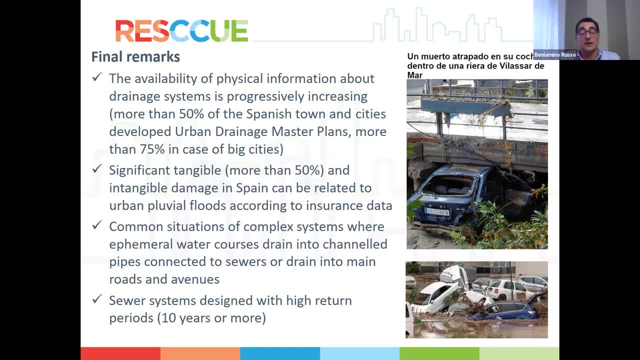 Okay, this is an information about the parcels, the polygons of the parcel, that is available from the cadastral organism that manage the properties in Spain, So you could access to this web page. Of course, you have to to proceed with the login etc. But you can download. 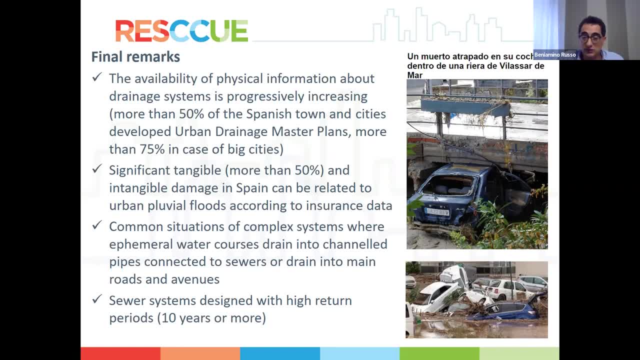 this information freely And we use this information on the polygons, the information about, for example, the age of the parcel of the properties, the number of basements, etc. So it's useful information for the economic damage model. So another question, like you know, for the economic cost that vehicle damage and all, 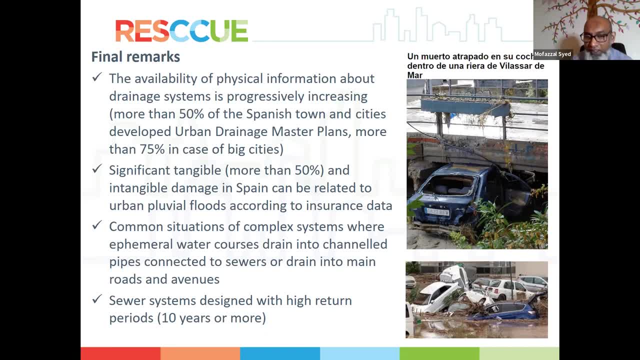 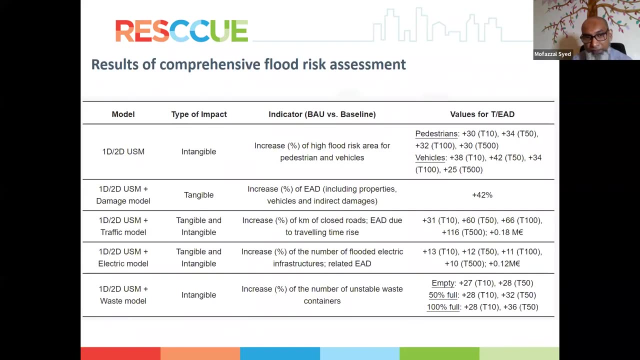 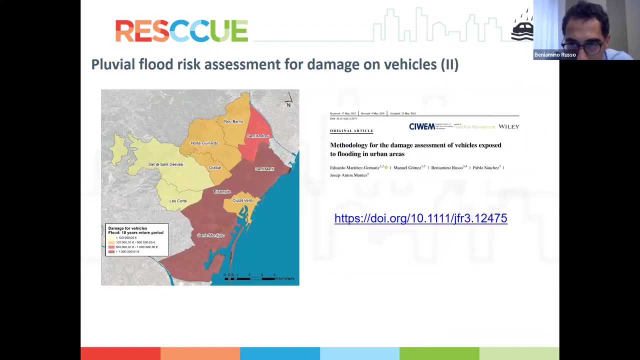 this. Did you compare that against the insurance database and how? if you do so, how did it compare your model prediction and the predicted cost and insurance claims? Yeah, The methodology for the damage assessment of vehicles exposed to flooding in urban areas. In these articles you can find: 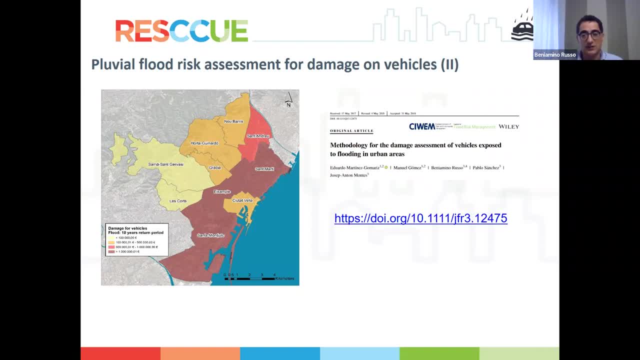 a tentative of comparison. Of course, in this case it's quite difficult to compare these kind of things, but we add the data. So for a specific event we have the data. in this case, not in Barcelona, but in Badalona, a city very close to Barcelona. This validation was done before the rescue project In an 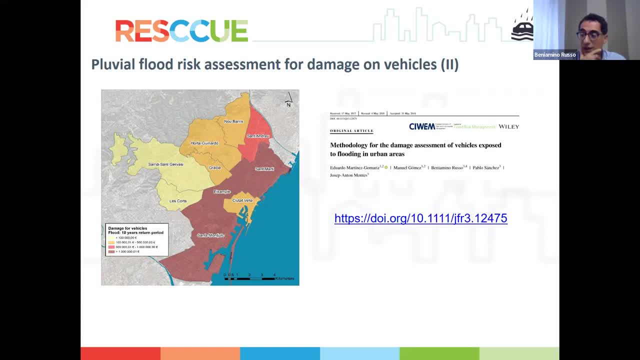 other European project, the Bingo project. We validated our results comparing the modeled damage to the historical ones. This historical data that I have cited before provided us damage not only for the for the parcel, but also for the vehicles. Generally are parked vehicles on the streets? 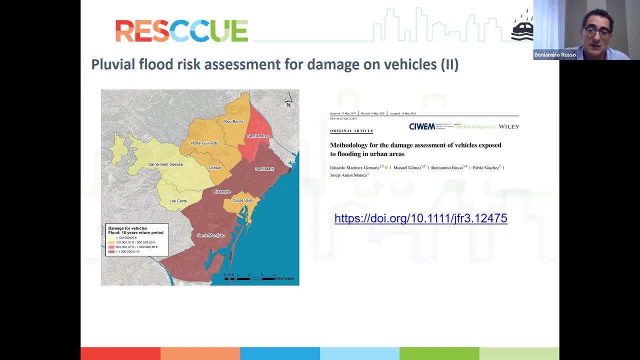 Because another thing is the presence of vehicles into the basement, into the underground parking. We are considering, in this case, flooded vehicles on surface. We removed all the noise, all the other data and we focused on this kind of data. Honestly, I think that we reached the same order. 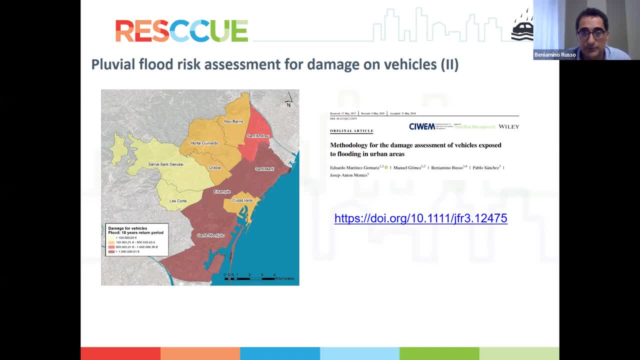 of magnitude, but it's a starting point. Of course, it depends on how the data is. You can see the publication, of course. Thank you very much. And one last thing, an observation: Great to see that you have been using the social media. 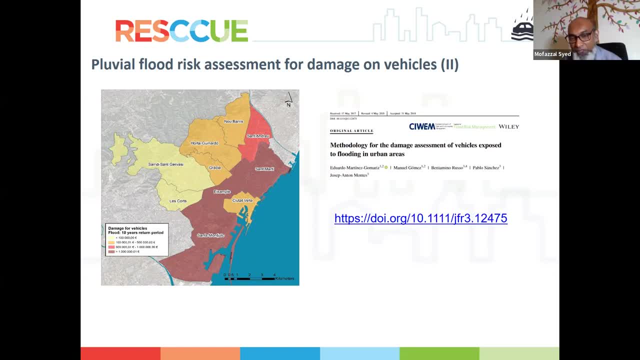 footprint to validate. And, on this note, I would encourage everyone, every participant here, to upload any flooding photo in urban areas, which is a great use for validating overland surface flow. And a question for you, Professor: How did you do the search of open source web data? 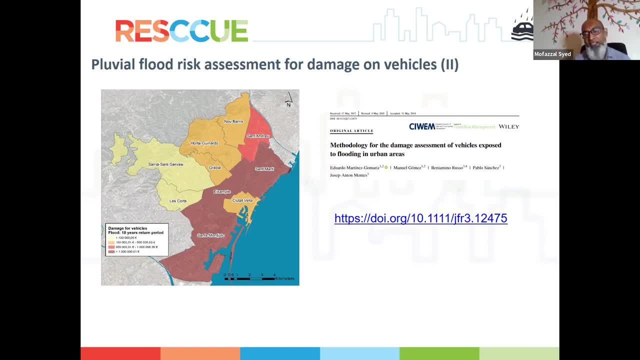 like social media data. Did you use any specific tools? Yes, How did you get on with that? A previous comment. I think that it's the unique way to replicate this kind of analysis in other sites. After Rescue Project, we developed this kind of analysis, for example, in Malta Island. 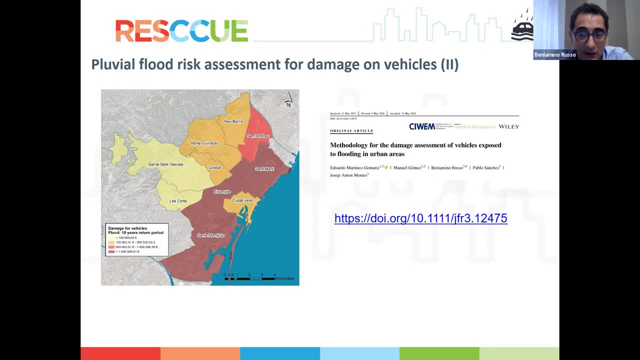 without severe flow meters, With very few rain gauge data, et cetera. So we developed the model using, let's say, the common sense, But then we needed the validation of these hydrodynamic models. The unique way to do that was the use of crowd media sourcing data. 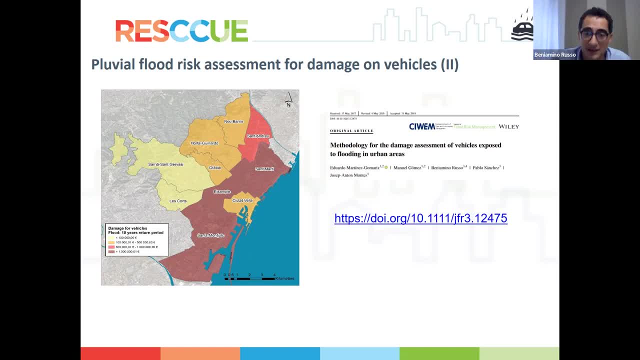 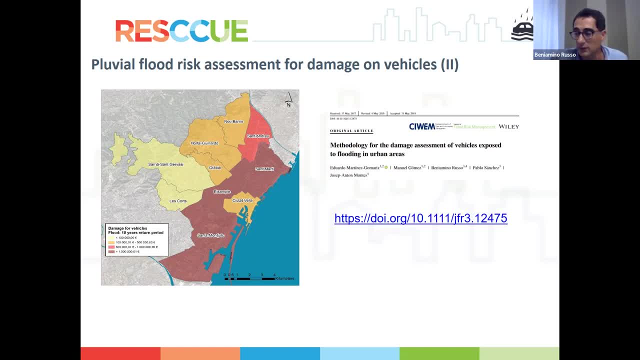 And we used a lot of data, For example, Google Map, information street map and very important civil protection reports. So no specific data. At least we are not so specialist in this kind of data. But I think that's it. 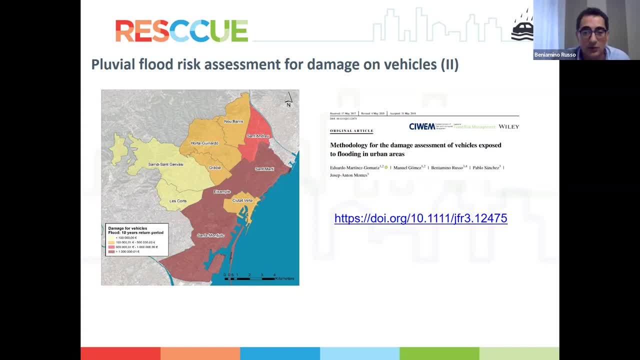 But I think that's it, But I think that's it. This is the way. This is the unique way to face with this kind of problem. So I'm mindful of the fact that we are heading towards the end of our time. So thank you very much, Professor. 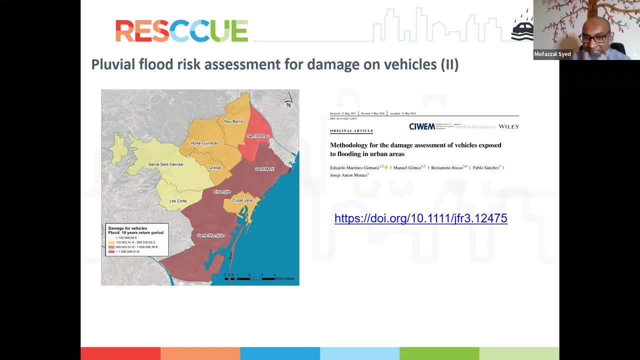 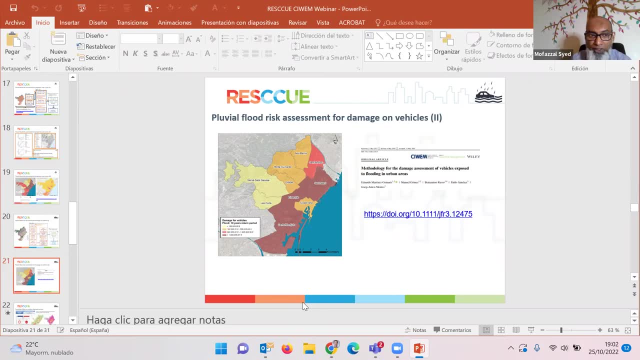 for giving us some time. It's good to know that what advanced research going on in this space And looking forward to get more of findings, Findings of your new project, And please let us know when you are in a position to present your findings with us.